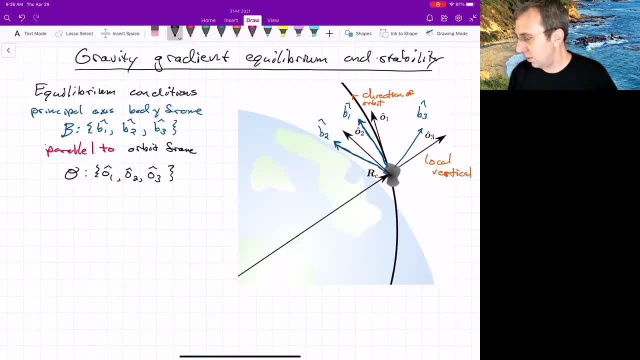 attitudes of equilibrium that are stable. it may be more than one. First, we have to get those conditions for stability. So we need to go back to what we had last time, just kind of setting up all the ingredients. we need to write Euler's equations right. This is what we want to do. 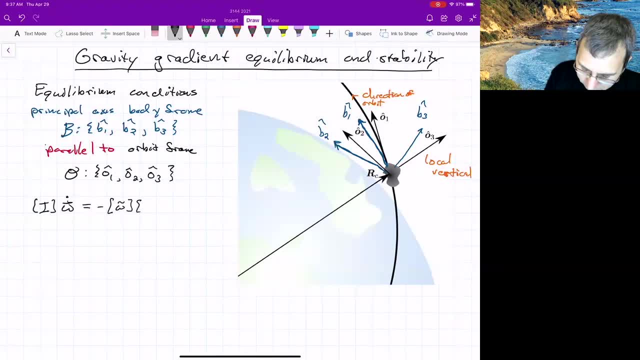 We want to write Euler's equations. We're writing it this way, plus LG. So equilibrium corresponds to omega dot. change in angular velocity going to zero. Stability will be something additional where there will be restoring torques, taking you at least not away from equilibrium, If you have a 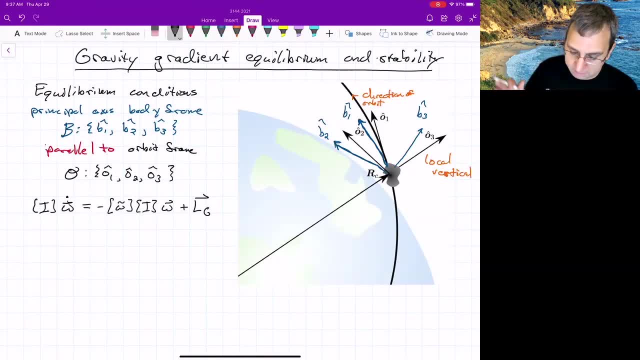 slight departure, let's say one degree. we don't want that to lead to instability. So all of the ingredients are not quite there. Gravity gradient in terms of the body: fixed principal axis frame: LG one, LG two, LG three, And this was three: G M E. That GM is what. 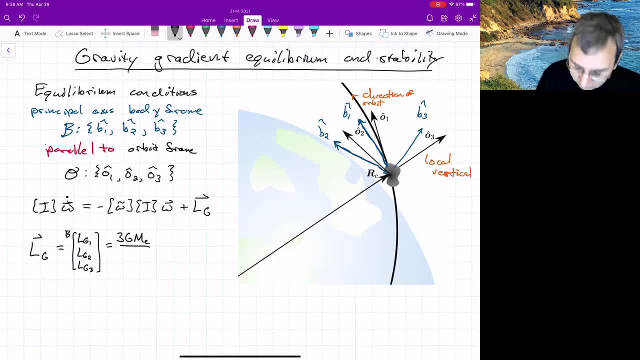 The Mu parameter, So it's something like 10 to the 14 in SI units, and then distance from the center of the earth. So that would be what the semi-meter axis, And then this combination of RC ones, RC twos, and then the moments of inertia. 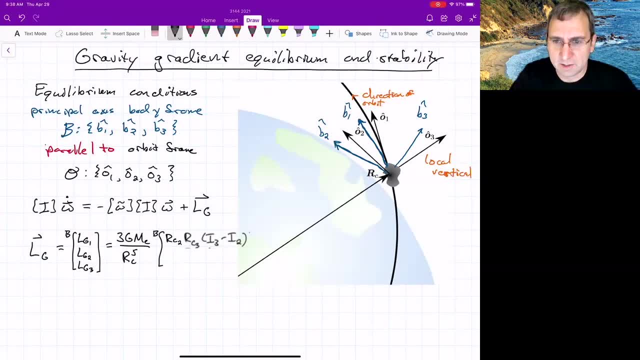 I one, it's along the B one axis, I twos on the B two and I three three. But then, for sake of clarity, we said that B three is definitely in the O three direction or it starts out near the O three direction, so that we can then start analyzing. 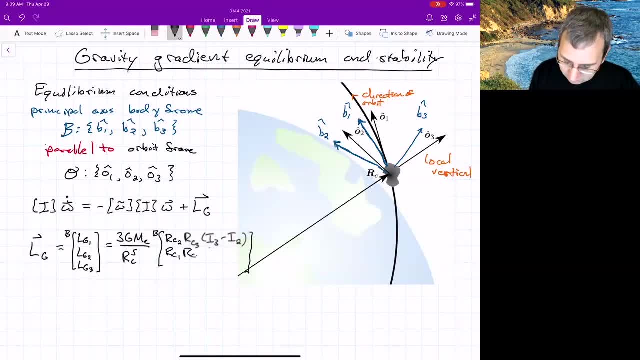 Next component was RC one, RC three, I one minus I three. And then the last one, RC one, RC two, I two minus I one. And what are all of these components? We're writing this vector distance from the center of the earth but, as seen in the body, fixed frame. 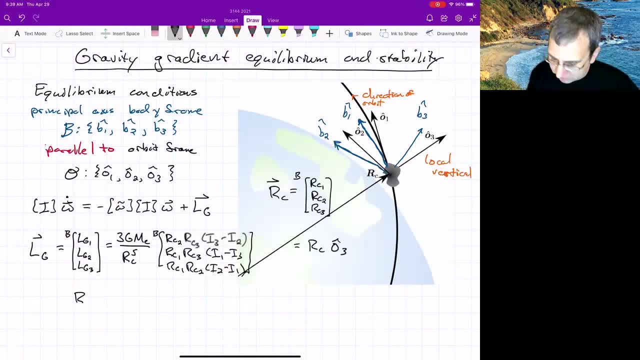 So this is RC, but in the O three direction, And we're just writing the components that result from that. I in the body fixed frame is, because it's a principal axis Frame- I one, I two and I three. We also wrote omega and omega dot in terms of Euler angles. 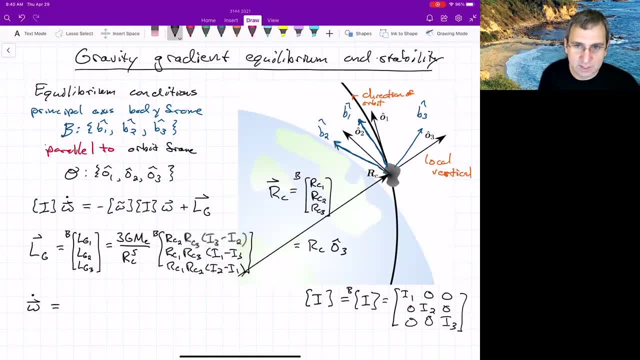 So omega dot how the angular velocity changes with time And this is approximate because we're making a small angle approximation writing in terms of yaw pitch and roll. So for example, the yaw angle is rotation about the O two direction. So if I were to draw it here, this would be. 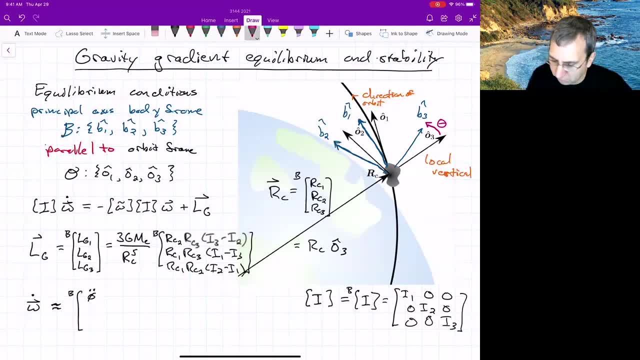 That would be pitch and yaw would be and roll would be other things. So we've got this. This is all again from last time, but necessary ingredients to do our analysis. We have that. And then we had theta double dot and we had psi double dot minus omega dot. 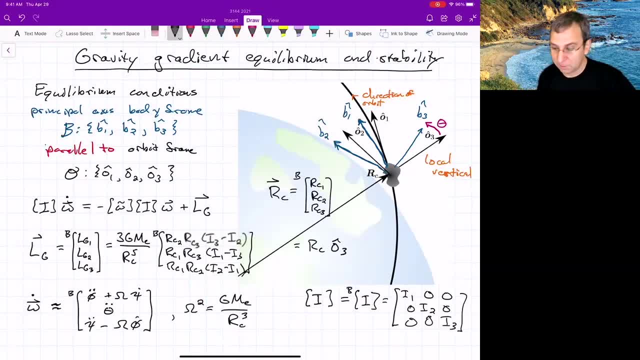 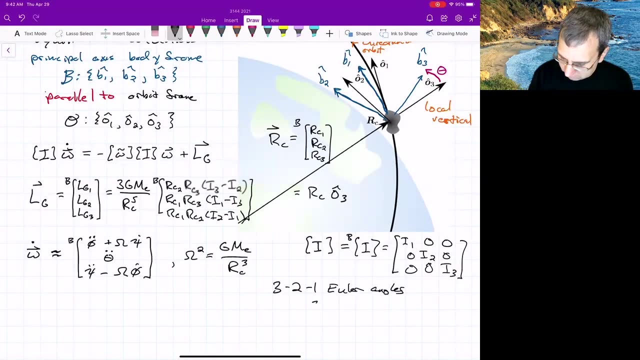 And remember this is just Kepler's law. Kepler's omega is angular rate. as we move through the orbit, and we're assuming a circular orbit, The analysis gets more complicated for elliptical orbits. but hey, more for people studying attitude dynamics. We can rewrite LG. We're using the three to one Euler angles: yaw, pitch and roll. 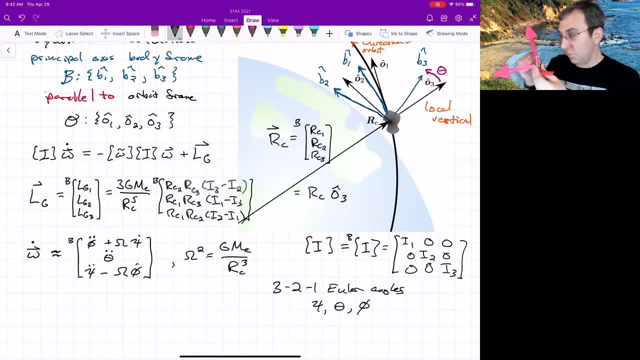 But assuming that the O frame, the orbital frame, is aligned with the B frame. So yaw is the same thing, It's rotation about that number three: direction, pitch and then roll is the last one. We'll see what else they offer us. 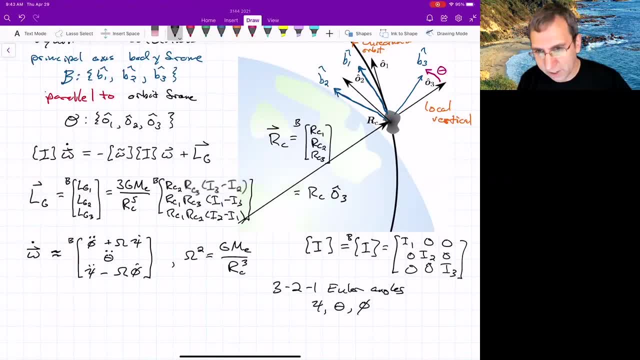 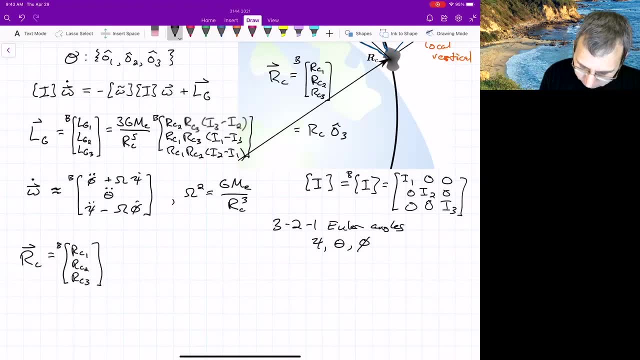 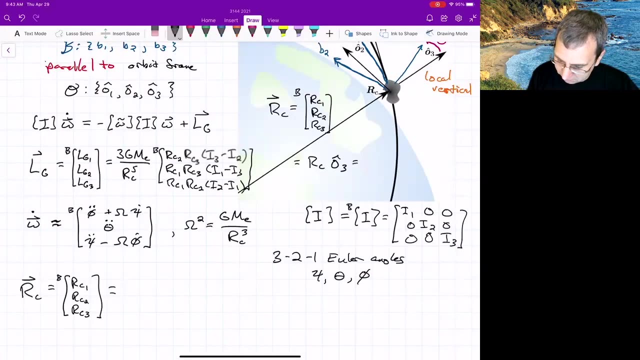 We have the, We have the. We want to write our C the vector. We won't write our C one or C two and 3 in terms of Euler angles. So our C rewriting it from their RC one or C two, Our C three, If we want to write this in terms of the orbit frame, and hopefully it's clear, right? This is the orbit frame, our C orbit frame: 01.. The beta O direction cosine matrix: Do, zero, zero, R, C, And this is just this tangent, right, right, And your tangent, this, the earlier end of it, and the çalentath and my tangent constant. 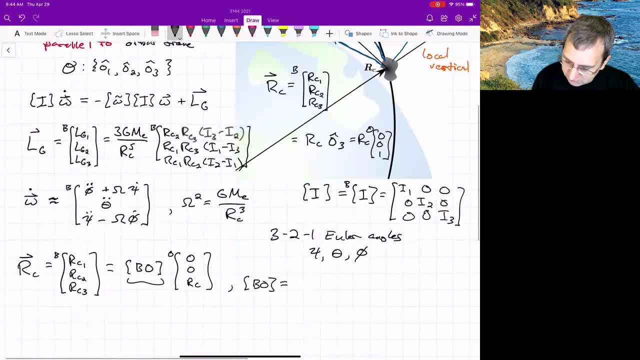 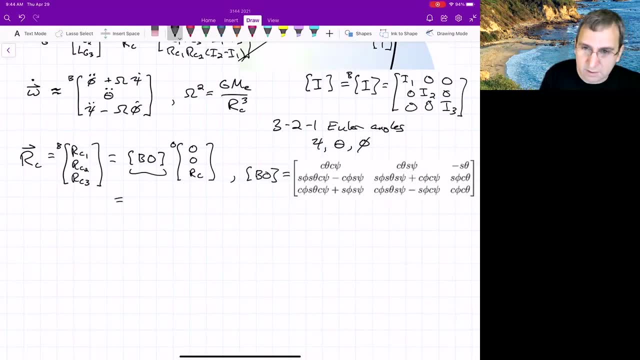 So R chose here to do a projection反ant method. And so now let me give you another expression right? the typical three by three rotation matrix, written in terms of pitch and roll angles, all right, so when we do that, you multiply through, then we get that this is the body fix frame, right? this is just 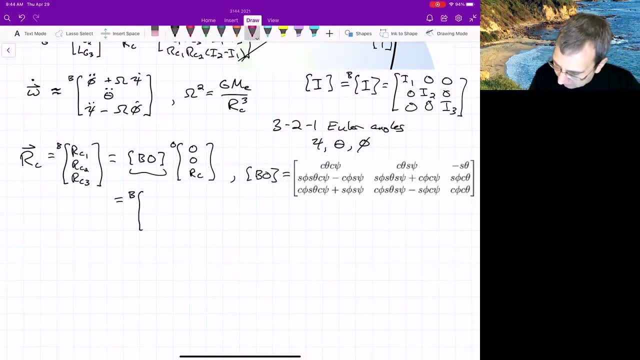 the o3 because it's the o3 direction. it means we're basically just picking out this third column. so negative sine theta, sine, phi cosine, theta, cosine, phi, cosine, theta times the scalar rc. so this leads to then lg what we wrote up above. we've got these components: rc1, rc2, rc3. 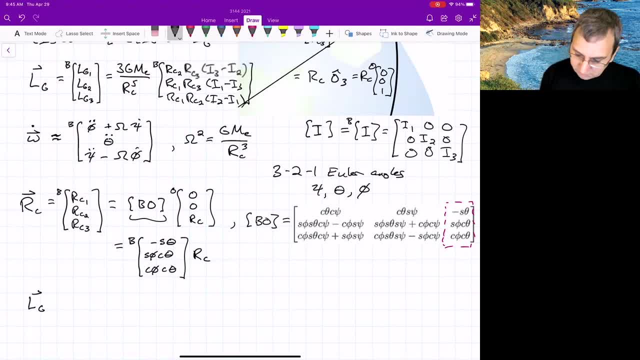 written in terms of the yaw, pitch and roll angles. so this simplifies. we'll actually get 3 g m e. we had rc to the fifth and then we'll get rc squared, so this will become rc to the third, and then i'll write this in terms of i3 minus i2 cosine squared. you collect some things. 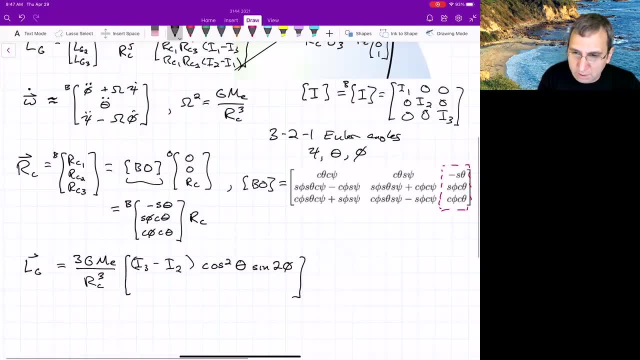 use a trig identity. this is sine 2 phi, and then the next one is minus i1 minus i3, cosine phi sine 2 theta, and then this is minus i2 minus i1 sine phi, sine 2 theta. there's a double angle formula being used over here and this is all in the b frame and you look at this and you go: oh. 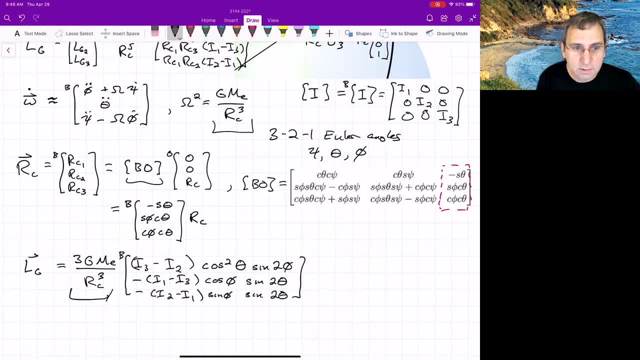 hey, what do you know? it's the same as this up here. it's kepler's law. we could just rewrite part of this term, this one as just capital omega squared. very nice notice. there's no dependence on yaw, which was psi. i've got my spacecraft and 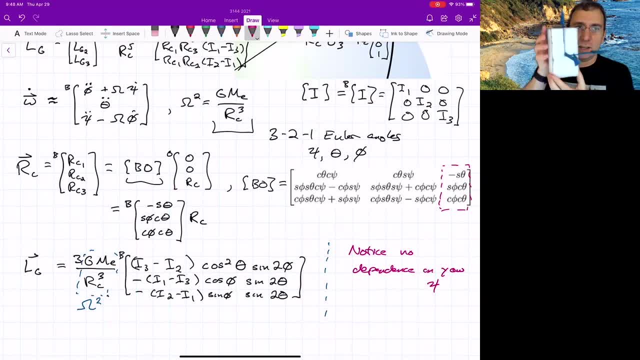 it's the local normal and this is the yaw direction. that yaw direction right does not affect the torque, only pitch and roll. and why is that? because that brings some parts closer to the earth and some parts further away, whereas rotating this way does not. so that's just something to notice. 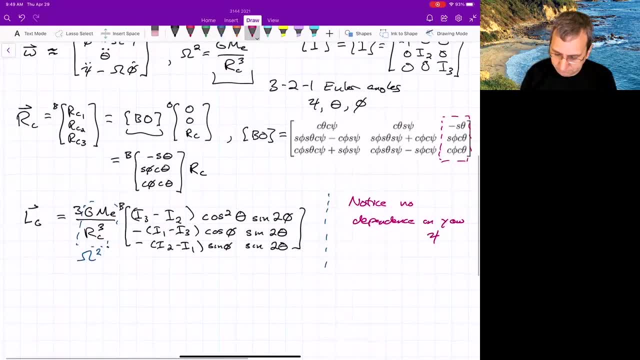 so if we now linearize this, i'm going to linearize about the zero, zero, zero configuration. so we're saying that that means we only keep terms that are leading order, just like last time. you know, cosine of something just goes to one, sine of something like x goes to x, and we drop everything. 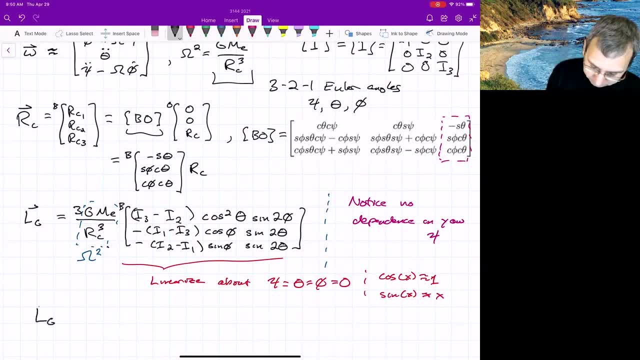 else. so lots of these things are going to drop out, which is good. Let me use squiggles. It's always fun to use squiggles. It's approximately three omega squared. This bottom term is just zero. So I like that. I3 minus I2 phi There. 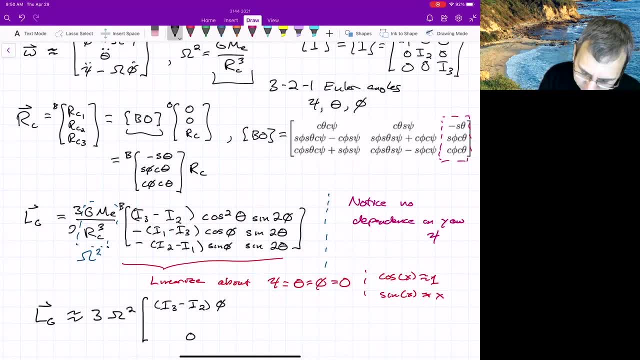 should have been like a factor of two somewhere. Yeah, I think it was a factor of two. Sorry about that, Because of the double angle formula. So then we would have two phi divided by two goes to zero. Okay, so this thing was actually three halves omega squared. There's a lot I'm trying. This is: 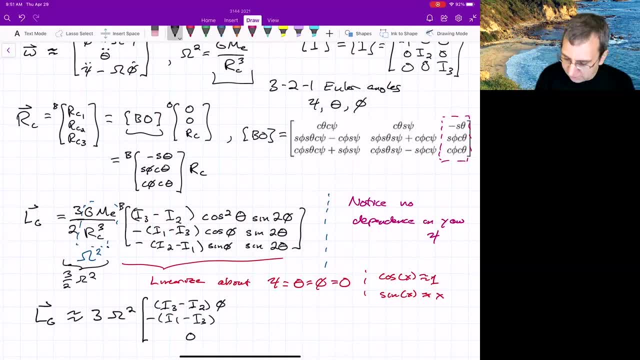 minus I1, minus I3.. As long as you get everything right before the mission takes off And notice the linearized torque will never even have a yaw component, No yaw component. So up here we were just noticing there was no dependence on yaw. And we're noticing here, linearizing there's not even. 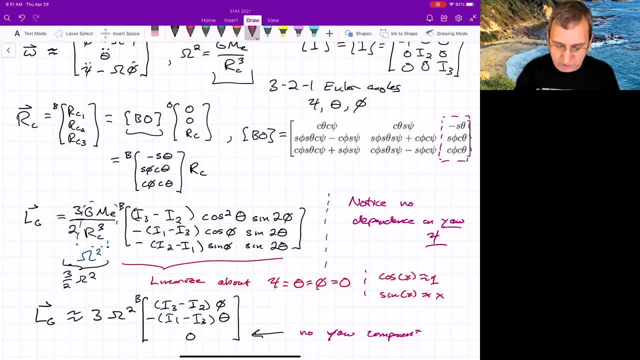 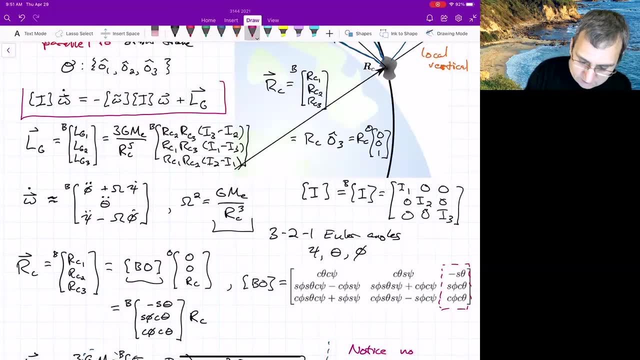 a yaw component to the torque- Two separate things. So now we've got everything we need to. if I sneak up here to now write this completely in terms of Euler angles and assuming small Euler angles. So for small yaw pitch and roll, There's still another step for linearization. 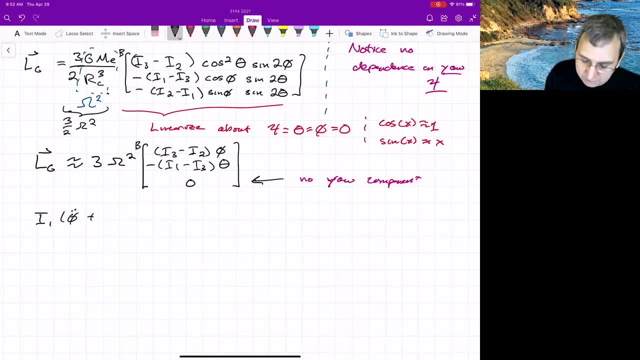 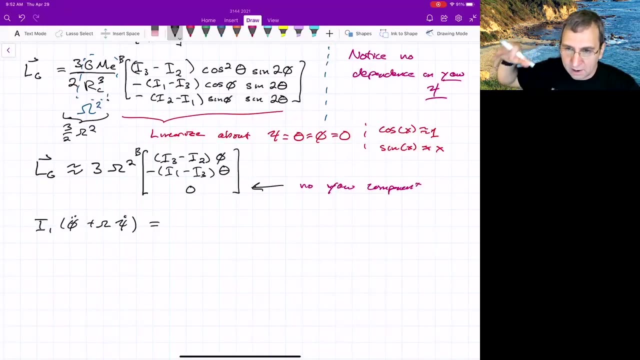 We'll have I1 times phi, double dot plus omega yaw dot. In that matrix equation it's actually three scalar ODEs. So we're writing those three scalar ODEs. Okay, the first thing comes from that negative tilde, I times omega And we get this from that. 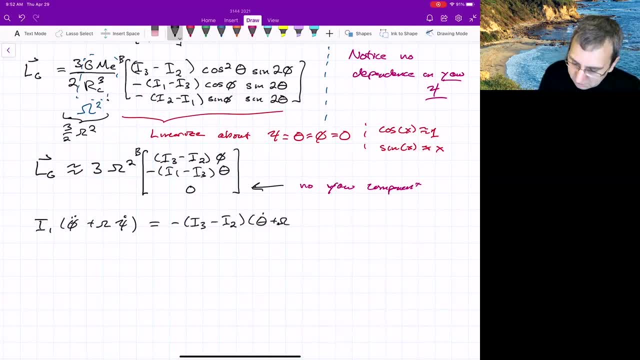 multiplication: Theta: dot plus omega psi, dot minus omega phi. And then the part that's due to the gravity gradient, which is three omega squared: I3 minus I2 phi. The others are equally bad. Actually, this one isn't so bad, And this is minus I1, minus I3. 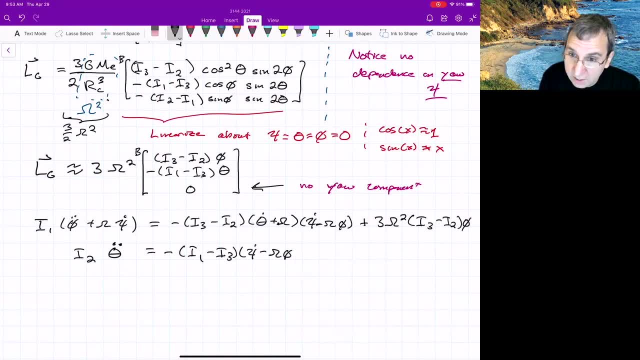 psi dot minus omega phi phi dot plus omega psi minus. So now we're putting in the gravity gradient three omega squared: I1 minus I3 theta. Okay, now we're I3 psi double dot minus omega phi dot equals minus I2 minus I1 phi dot plus omega psi theta dot plus phi, And there's no. 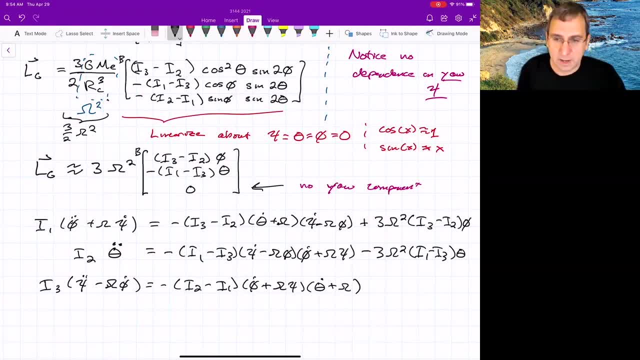 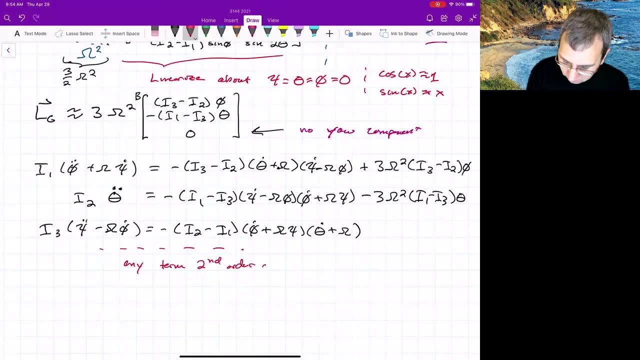 component due to the gravity gradient. Now these expressions contain products of angles and angular rates that we're assuming are small, So these equations can be simplified further. So any term second order Or higher in small values, And we're assuming that you know the roll, pitch, yaw and their 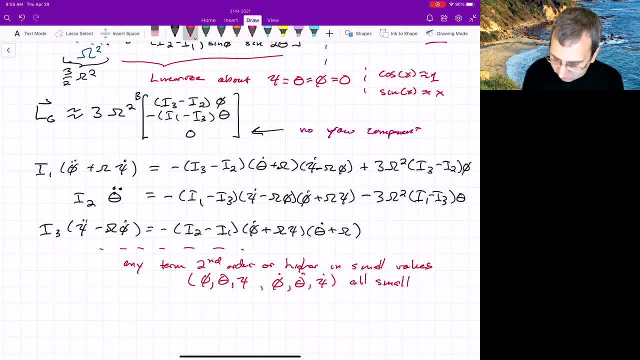 rates are all small. Anything that's second order higher in that we just neglect. Basically, we set it equal to zero. Look at this pitch equation, pitch equation. right, We'll have this multiplied by this, that'll go away. We'll have this multiplied by this, that'll go away. This: 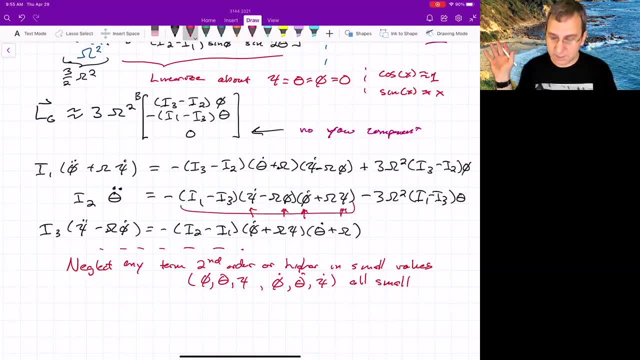 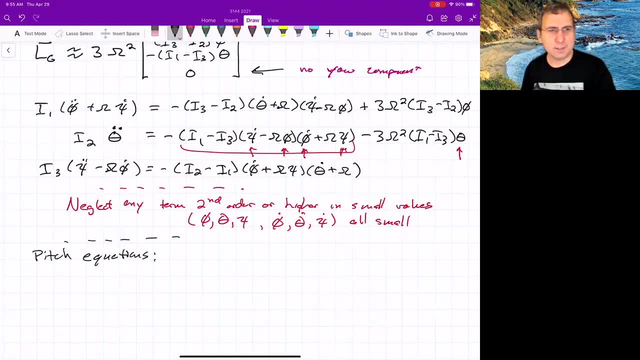 multiplied by this. So this, this whole thing, is just going to go away, And then we're going to go away because it's all second order. Over here, though, we got something that's first order, So maybe look first at the pitch equations. Anyone hear like a instrument in the background. 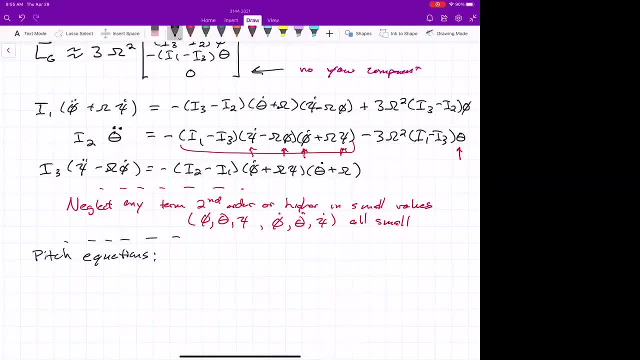 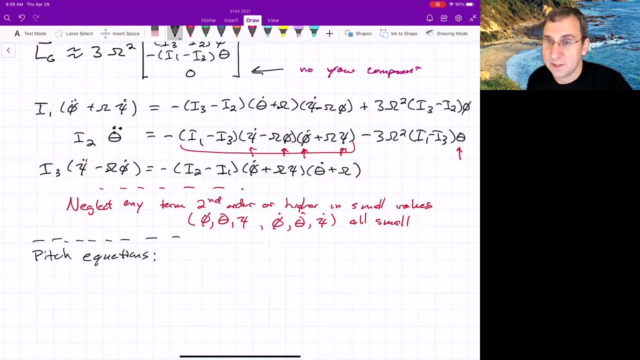 I hear something I do. It's my son practicing saxophone. I could tell him to stop, But no, maybe it's kind of the atmosphere. Yes, it's like jazz. This is improvisational derivations, So he could do his improvisational. 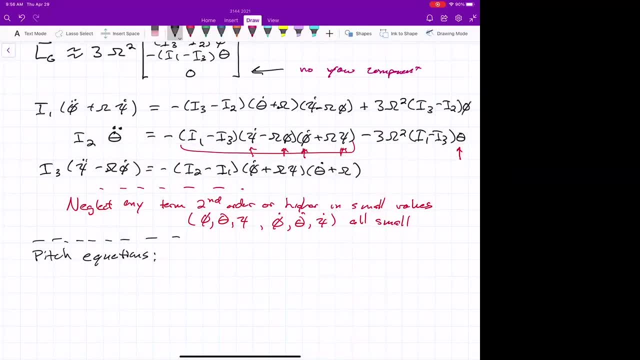 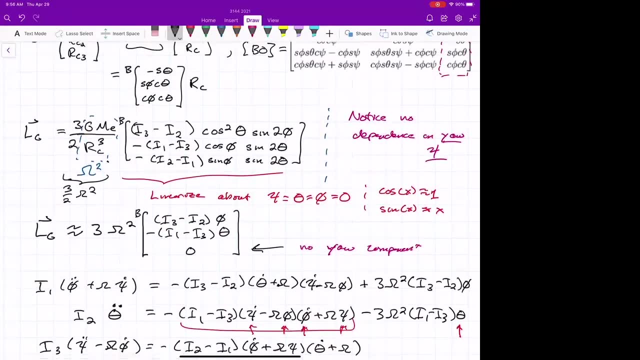 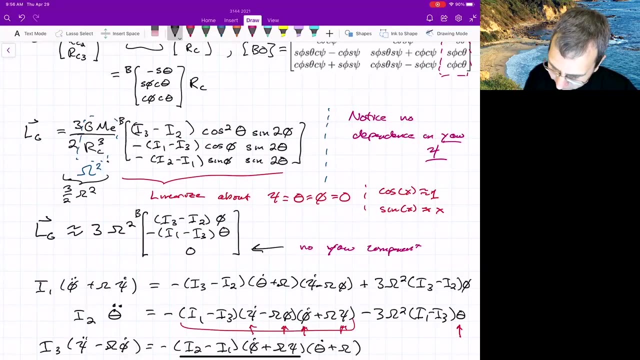 saxophone. I have a question. Yeah, go ahead. So above that LG equation you had. you had originally written three halves omega squared, but then that doesn't really carry down through. I was wondering where that one half term. Oh yeah, yeah, I hear you. So sine of two phi is approximated by two phi. 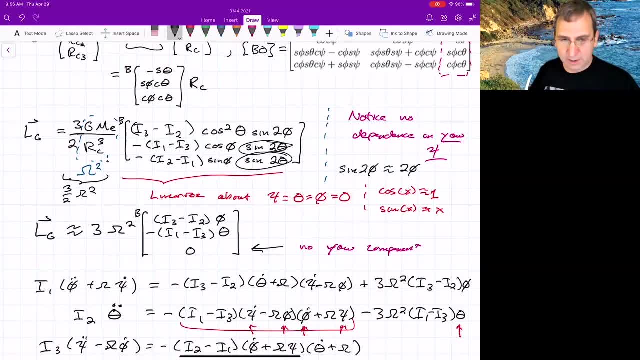 Ah, okay, Same for this. So all those twos. then come on out and cancel. Okay, Gotcha, Okay, Yeah, Cool. So the factor of one half came from the double angle formula, and then the small angle formula brings back the two and it's gone. So yeah. 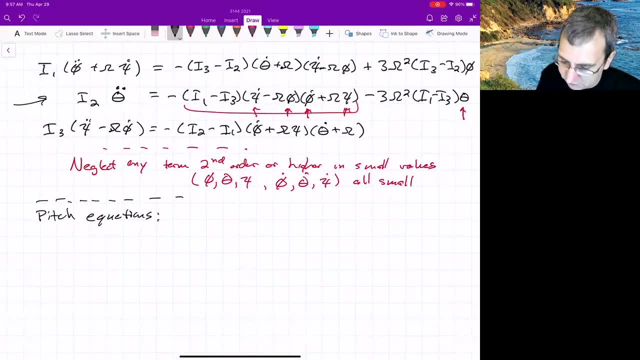 So we're looking first at the pitch equations, because this sort of middle term I've highlighted in red, it's got all second order and small things. So it will. those will all go away And what we're left with is, I'll put it this way: All right, I did not mean to zoom. 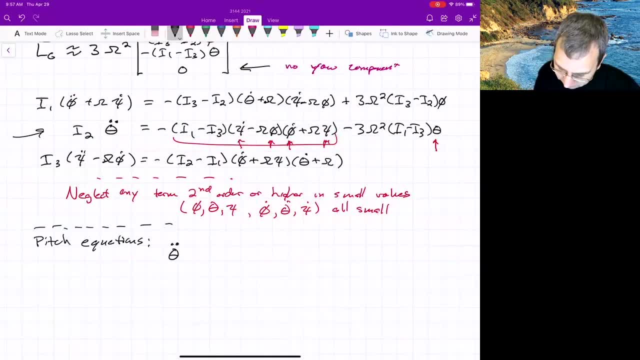 I'll put the I2 to the other side. I'll bring everything over. So this is theta double dot plus three omega squared: I1 minus I3 over I2 theta, And so now this should be highly recognizable as things that we've seen right. This looks exactly. 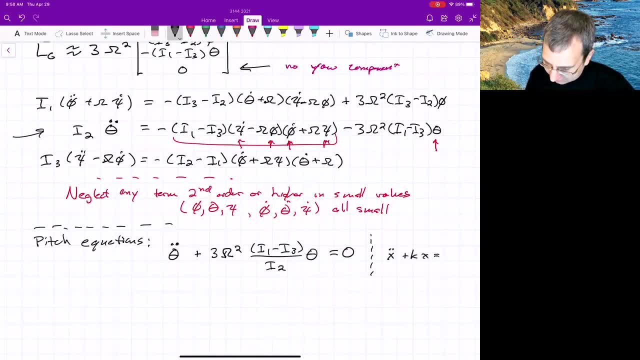 like X, double dot plus KX equals zero And you need K greater than zero for stability because that means it'll be a restoring force. It'd be like a positive stiffness for a spring If you had negative stiffness for a spring. the further you get from equilibrium, the further it wants to go. mathematically we have a. 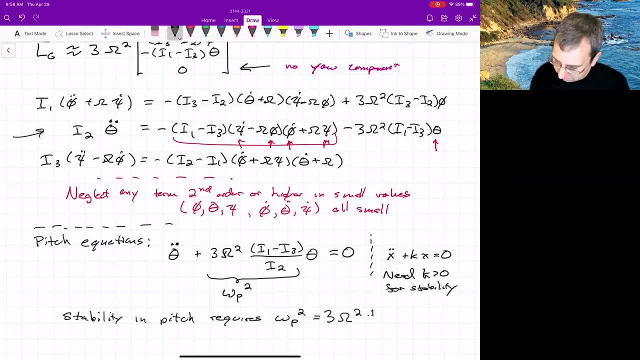 condition now for at least stability and pitch. Maybe let's call this omega P squared. Stability and pitch requires that omega P squared, which is three omega squared, i1 minus i3, over I2 greater than zero Omega squared is the maximum for same-��ging forces. 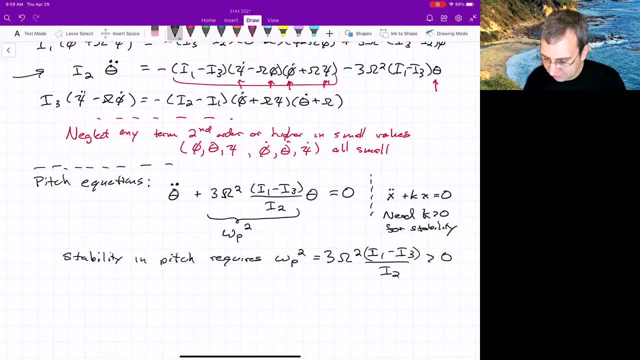 For each mitochondrial in an egg, Brigham, brigham, Brigham, Brigham, Brigham becomes a definitely greater than zero i2. all of these things. i1, i2 and i3- all of the moments of inertia- greater than zero. so this means that we need i1 greater than i3. now remember in terms of: 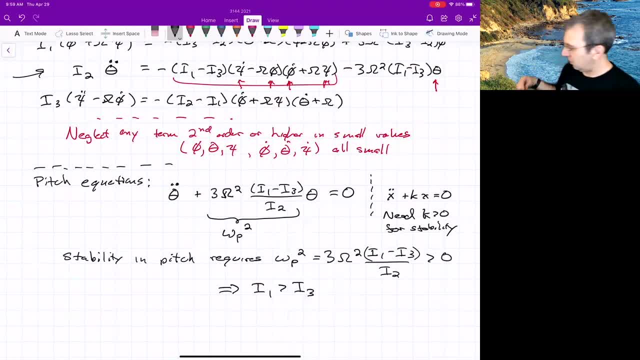 the orbit frame, i'll bring up the earth, earth. okay, so there's some orbit frame, orbit frame. now you can't even see it. there it is. this is the direction of the orbit, this is the vertical and this is the normal to the orbit. let me just show. 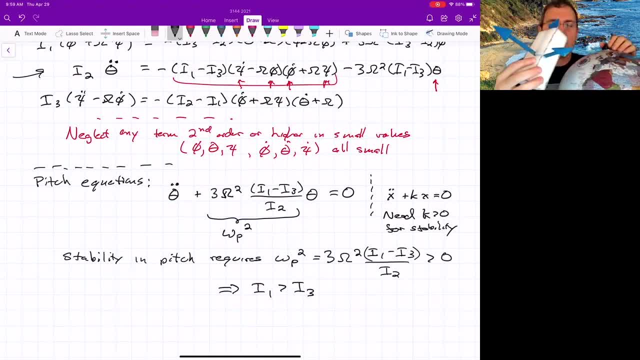 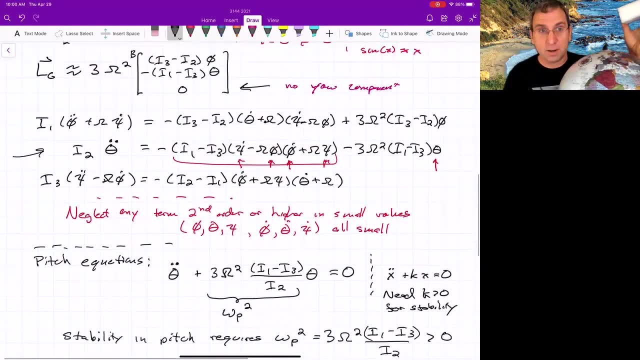 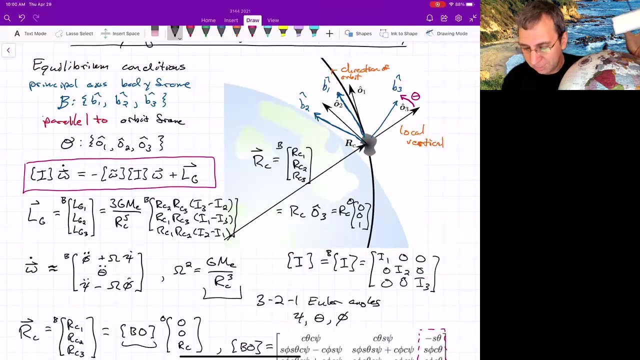 something next to the earth. so we need that. i1 is greater than i3. if we go back up here, i'm just going to show the orbital frame. so the moment of inertia about i1 needs to be greater than the moment of an inertiel wi't. so the moment of inertia about i1 needs to be greater than the moment of inertia. 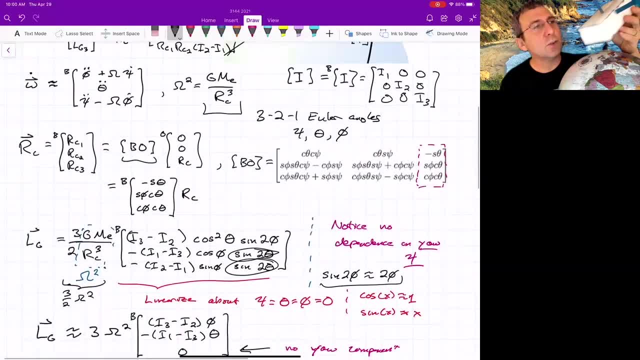 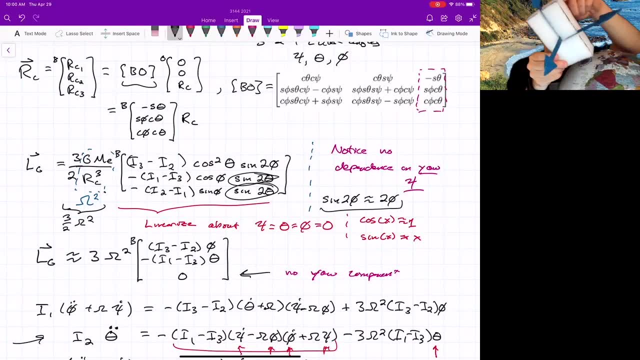 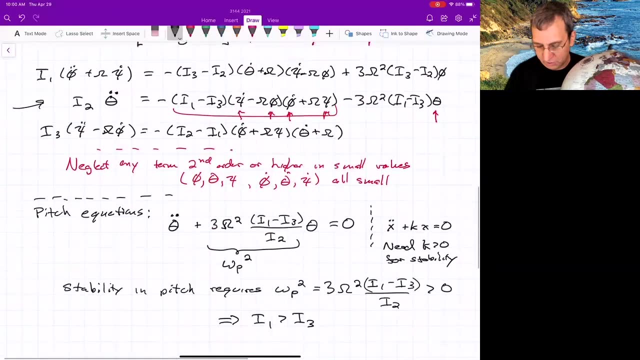 inertia about the number three direction. So what would that mean? That would mean we could have, if this is the Earth, I could have the kind of long axis pointing away And that would be greater than in the O1 direction. That's just for stability and pitch. We should probably say some more things. 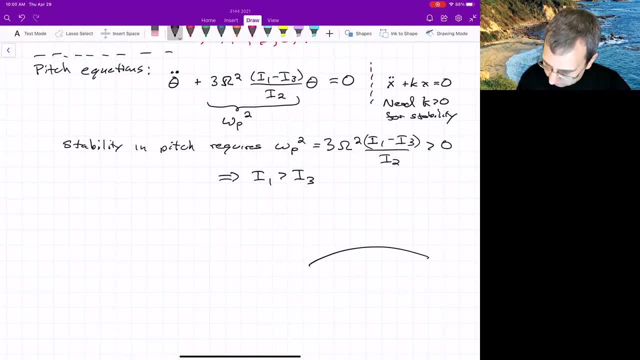 about pitch. Let's just give a picture. Here's the Earth And I'll do a side view. So this is the orbit frame, our local normal. It's O3. O2 is coming out of the screen And then O1. The 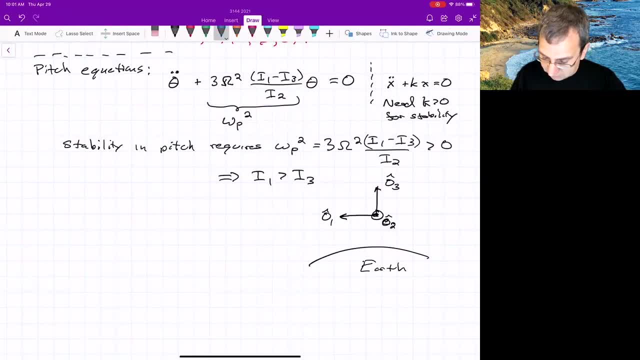 moment of inertia about the O1 axis. So that means we need a lot of mass kind of normal to the O1 axis compared to the mass that's normal to the O3 axis. That would lead to stability, And if you were to tilt this somewhat, there'll be a restoring torque to bring it back. So this exactly. 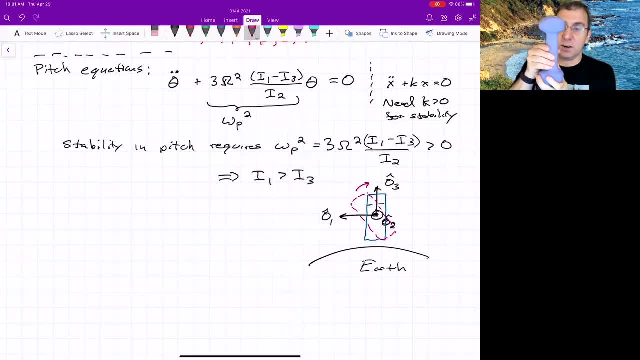 matches. Hopefully the intuition about the dumbbell. You've got a really large moment of inertia about this O1 direction, Small about O3. So if it goes this way it's going to restore. If we had it this way now we've got something really large in the O3 direction and something really small. This is 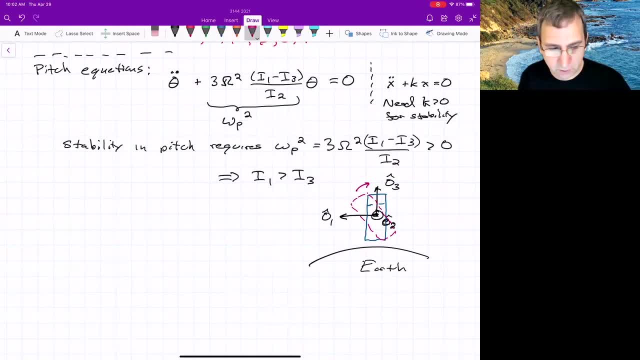 unstable. So think of the dumbbell or your phone. Here's your phone orbiting through space. You could do this, You could do this. Those would both be stable in pitch. I wonder how many phones are floating. I want to say some other things about pitch, because it is notable what happens in this. 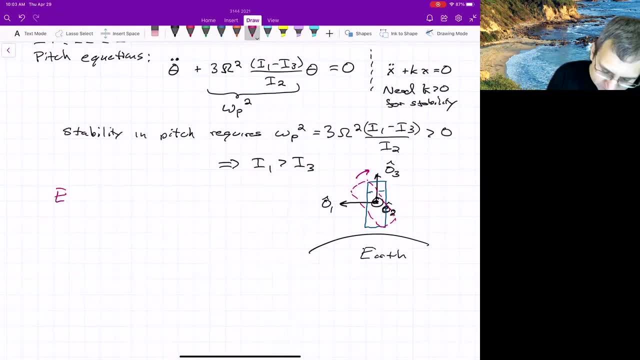 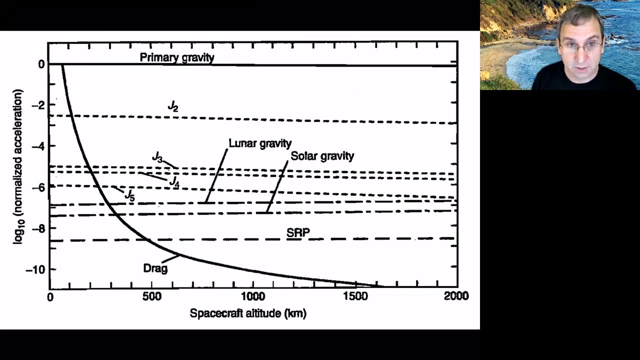 direction when you are close to the earth, So low altitude. there's environmental forces and torques. We've gone on and on about one of the main ones, the torque due to gravity, but there are others. This is showing the accelerations right. Forces per unit mass on the spacecraft, a different. 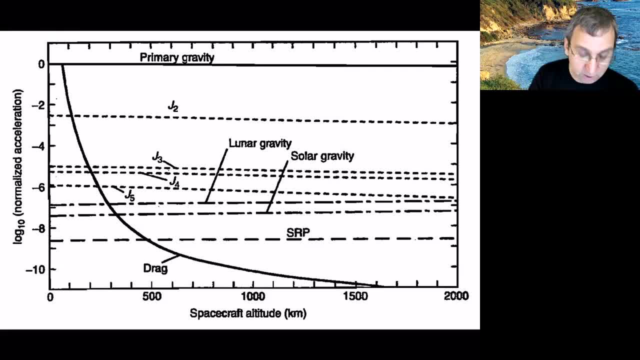 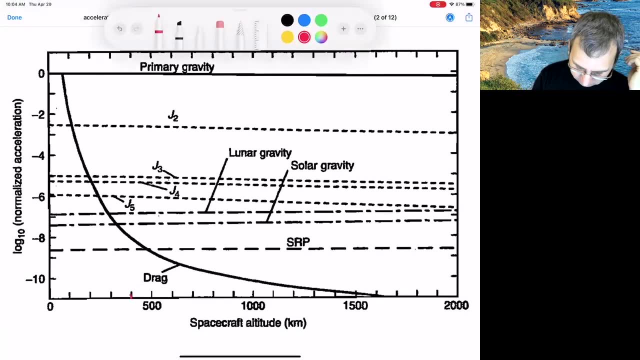 altitudes. So there's the primary gravity. This is a log scale, vertical scales, log. so primary gravity is like the top and if we're at an orbit of like 400, which is you know where the space station is. so for right here you can kind of follow this up, see what are the major forces. 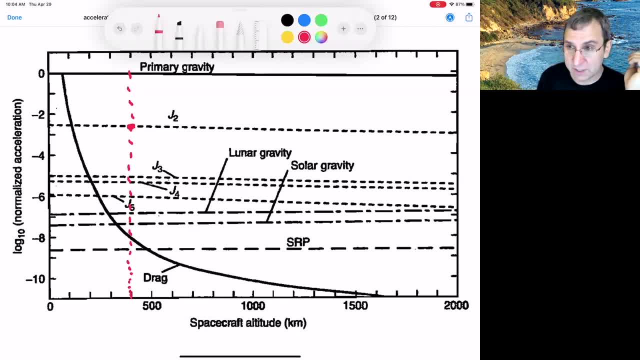 j2, j2 doesn't affect torques, at least not on the time scales that we care about. and then there's all these other: j3, j4, j5, so these are related to the distributions of mass in the earth. but then you get down to drag. now, actually drag can be. it's a lot more uncertain than this plot lets on. 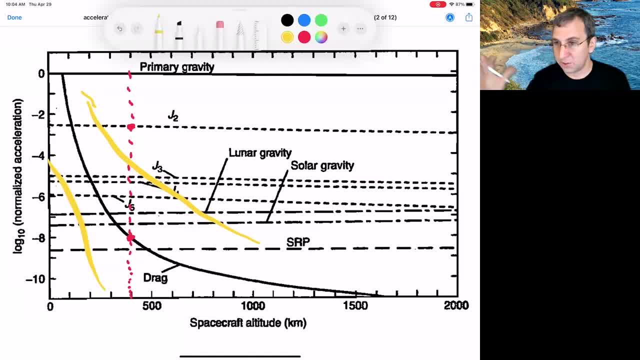 it depends on your exposed projected area in the direction of your orbit. so even up at 400 kilometers, there's enough of an atmosphere to create an aerodynamic torque, even if it's not a major contributor to the orbit. for large things right, like the space station, this leads to. 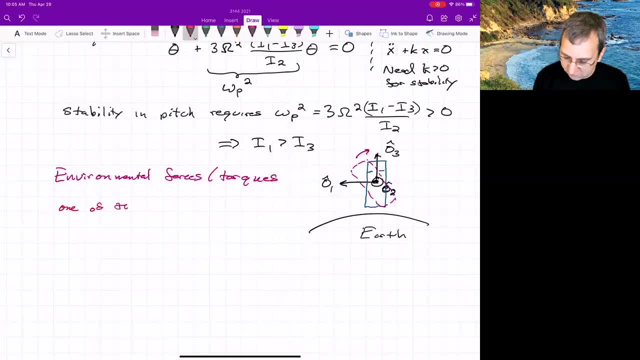 degradation of the orbit, but the the effect that we care about is the effect on the torque. so one of the main ones is the aerodynamic torque, and we might just write it this way. i'm not going to go into the details of how to compute it. it is related to that projected area, but it's good to know that it's typically not zero. 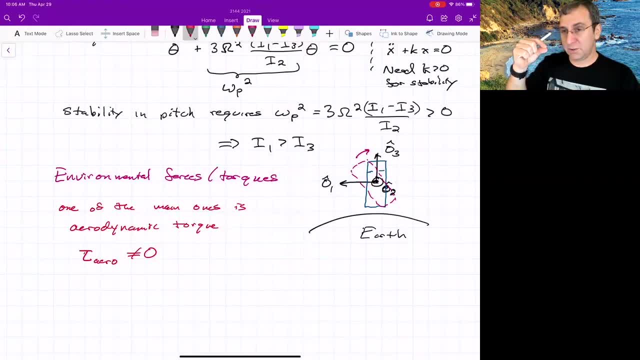 it depends on where the center of pressure is in the body compared to the center of mass. so if i'm going through space and i have a center of pressure here, then that's going to lead to like torque downward, but of course that could be balanced by the torque due to the gravity gradient. 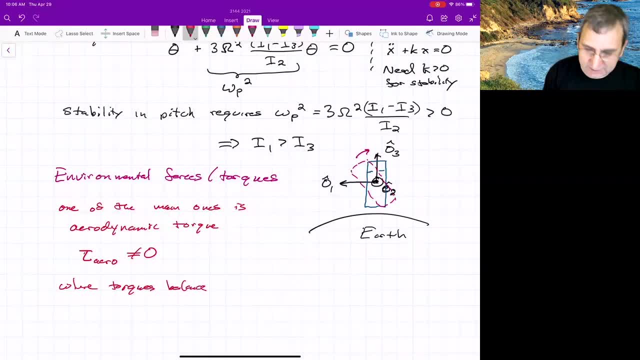 so, basically, where you'd want to be the center of mass, you'd want to be the center of mass if you're torque's balance. This leads to a deviation from the zero pitch condition. Torque's balance one gets T-E-A torque equilibrium angle And it could depend on how you're deploying solar. 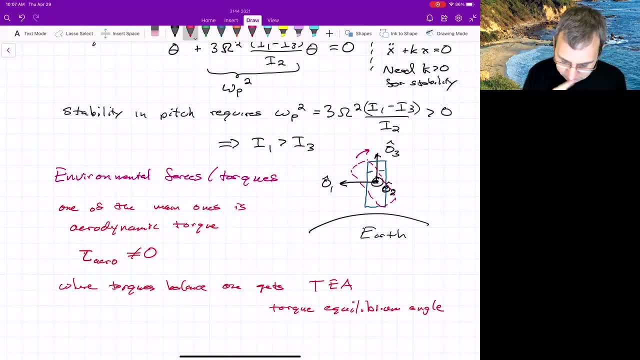 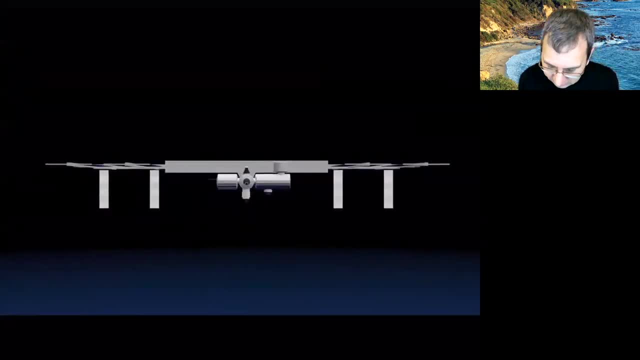 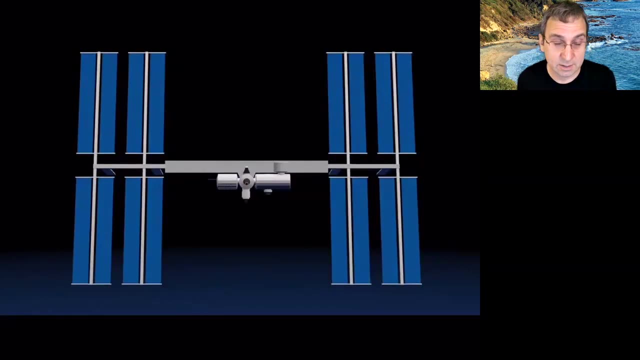 panels and things. So if we try to understand this in terms of the space station, here's the space station in a side view. So orbit is going. So now we're looking at it from the direction of how it's orbiting: right As it moves those solar panels, that gives an increase in aerodynamic. 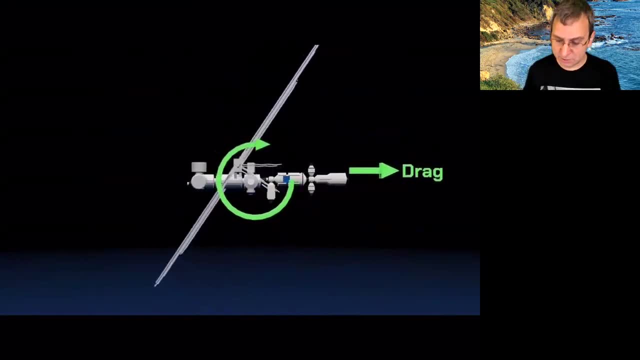 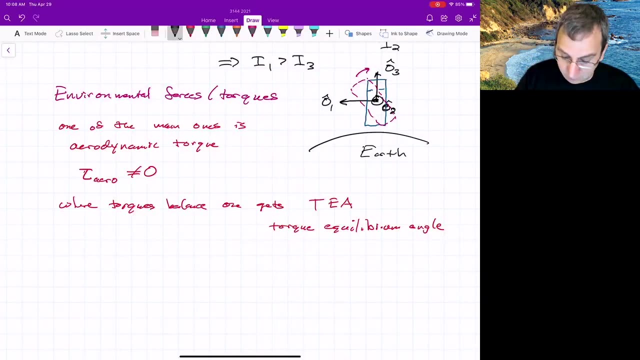 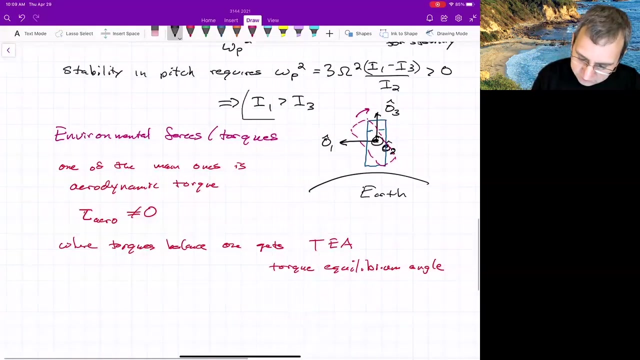 torque. They don't have much mass, so they're not changing the mass distribution, but they do lead to increased drag torque. All right, so there's the torque balance. I want to give you an idea, because this determines the torque equilibrium angle. If we're in this condition, where there's 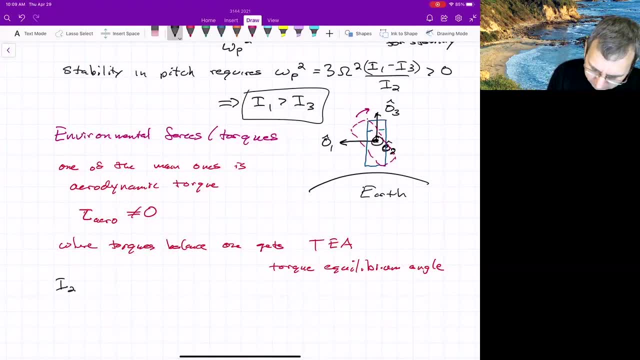 stability. let's go back to that torque equation I-T, theta double dot. This is the torque equation for pitch. Why are we focusing on pitch? Pitch is that angle of deflection that's going to be affected by any kind of aerodynamic torque? 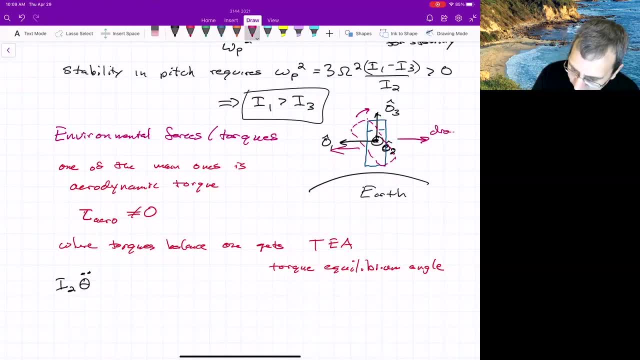 If our orbit is going this way, then drag is going to be going that way And it's mostly going to be drag. I mean, maybe there's some component of lift, but we mostly worry about drag And even small drag over many orbits. And you're going really fast, right? You know the formula for. 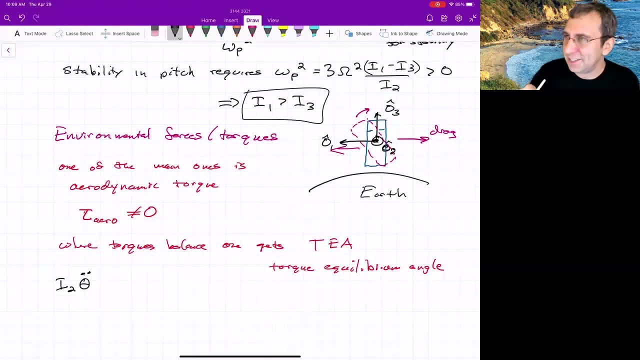 drag. It's like density times velocity squared And you're like: well, the density is small, Yeah, but velocity is immense, so it could be significant. So what do we get here? We get minus three omega squared: I1 minus I3.. And now let's add in that there could be a torque due to. 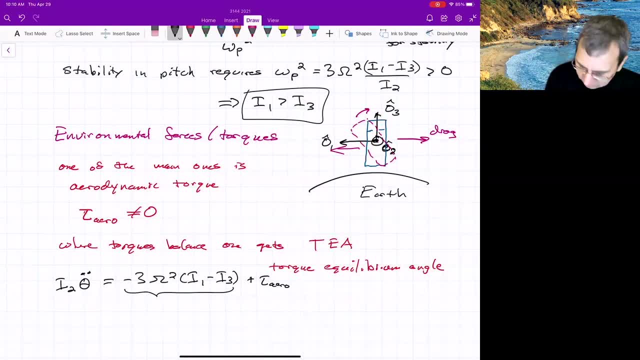 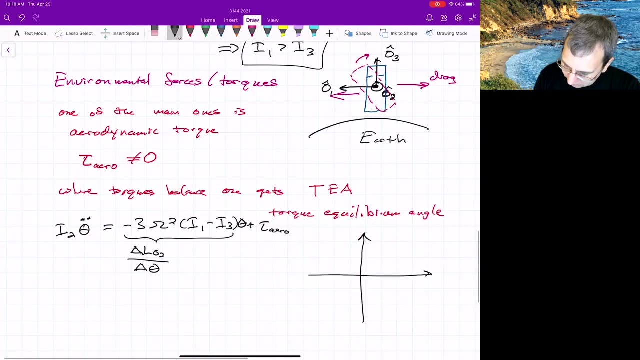 aerodynamics. We've been calling this what LG. So this is like LG2.. Oh wait, I need to put in the dependence on theta. I'm going to say this is delta, LG2, delta, theta. If we were to plot for the stable condition I1. 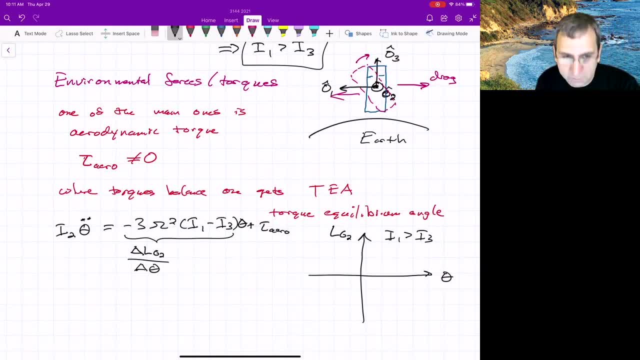 greater than I3, plotting LG2, but only for small theta. For small theta, this will be a curve that goes down like this: How do we interpret this? If we're at a positive theta, we have a negative torque, So it's actually restoring us back. If we had a negative theta, well, now we have a positive. 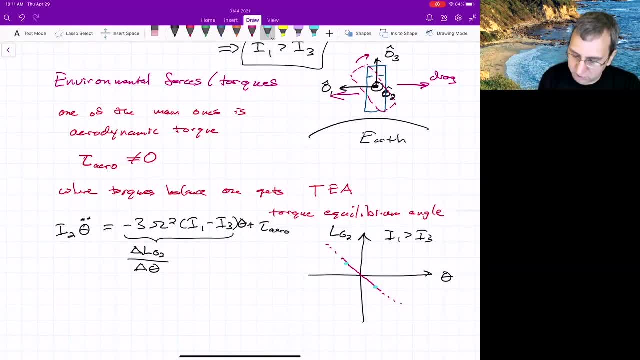 torque, again bringing us back In terms of figuring out where the balance point is. so for this we have what Delta, LG2, delta, theta is negative. It's restoring. If this was torque, then think of right here would be the negative. 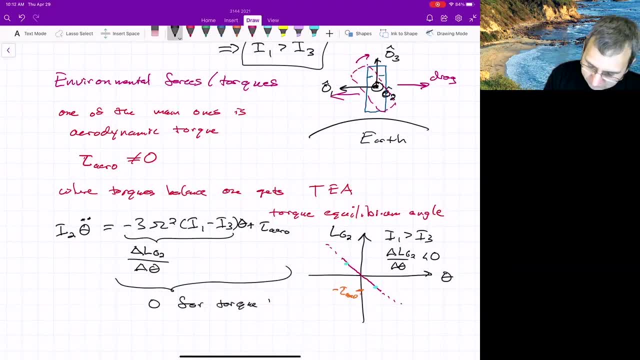 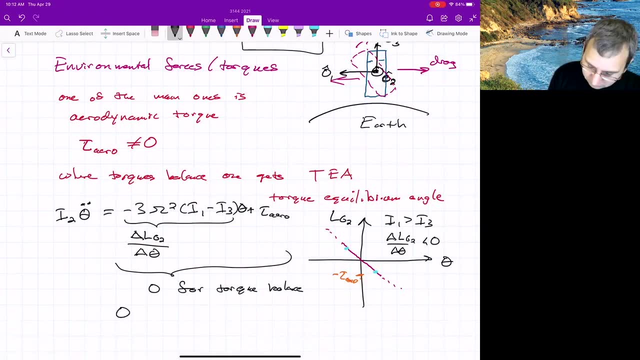 of our torque. For torque balance we need that this right-hand side is zero, And that's what we'll call our equilibrium angle. So set this to zero, And then we're going to do this, And then we're going to get this equal to zero. We've got theta. torque equilibrium angle equals negative. 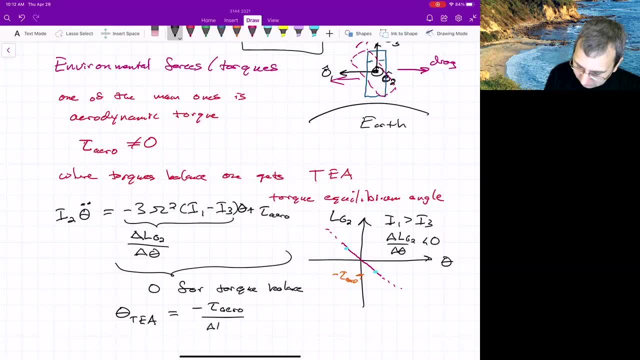 the torque due to aerodynamics, divided by delta, LG2 delta theta. And what was delta, LG2 delta theta? It is negative three omega squared: I1 minus I3.. So once you get that, you could figure out what the equilibrium angle is. And then we're going to do this, And then we're going to get this. 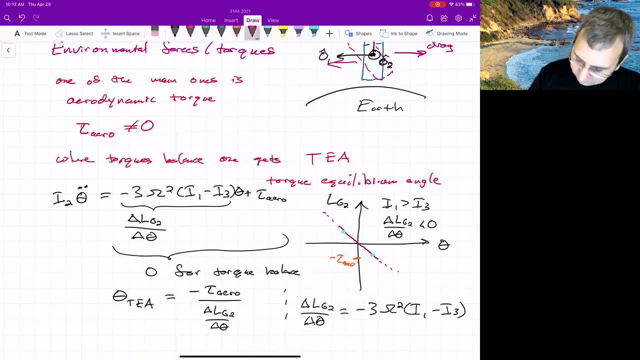 angle is, if you know what its moments are. I think if we were to follow these curves out further right- And this is always in radians- We've got to do this in radians- It reaches a maximum and then goes back down, But we're only looking, we're kind of linearizing about zero. 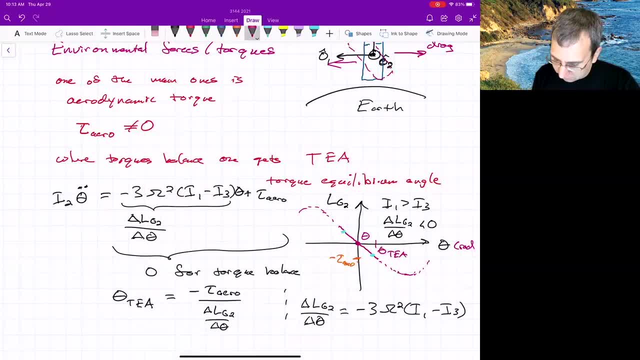 So then this would be the theta torque equilibrium angle For this case. if we had a destabilizing torque, the aerodynamics might actually stabilize it. Okay, So that's enough about pitch. We've said what we need to know about pitch. So if you're asked, what are the stable? 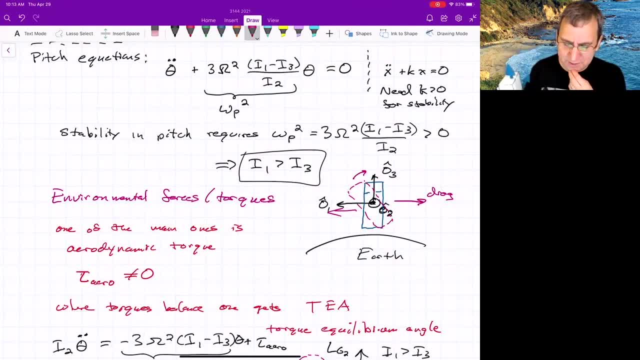 we haven't yet figured out completely. We know that I1 needs to be greater than I3.. We don't know where I2 fits in. Is it greater than I1? Is it between these two? This is the square of your frequency and you need this greater than zero. So you need this. So this is the period of. 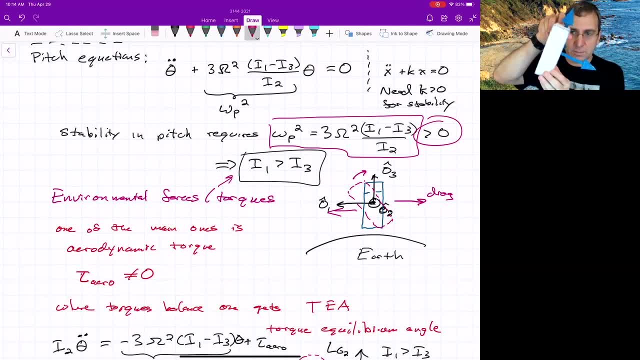 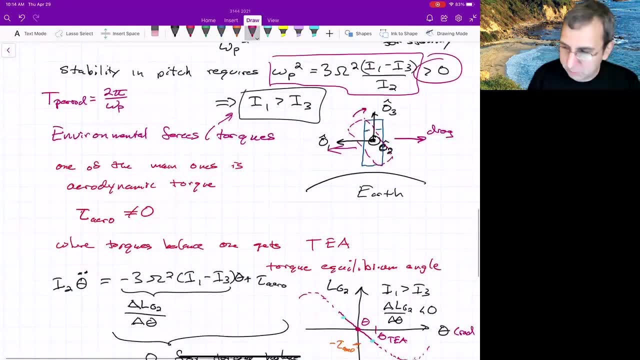 oscillations. If you start out with a little bit of a perturbation, there'll be these oscillations in pitch, which would lead to then periods of pitch And hopefully everyone knows how to. So that was for pitch. Yaw and roll are not as easy. 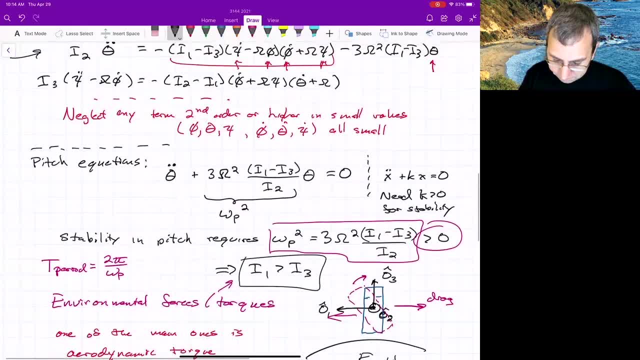 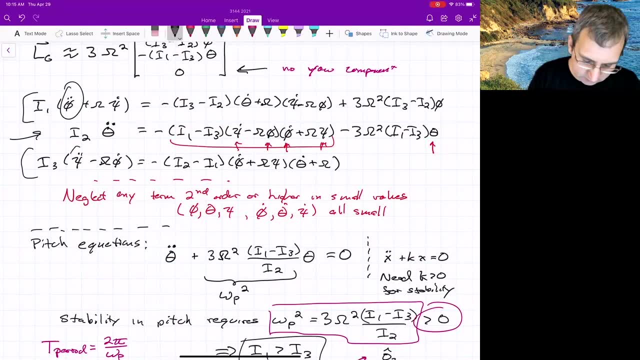 If we, I guess I need to go back up here to see what's going on. This is the roll, And this is why do I call this roll, Because the second order derivative is roll. And then this is yaw, And we. 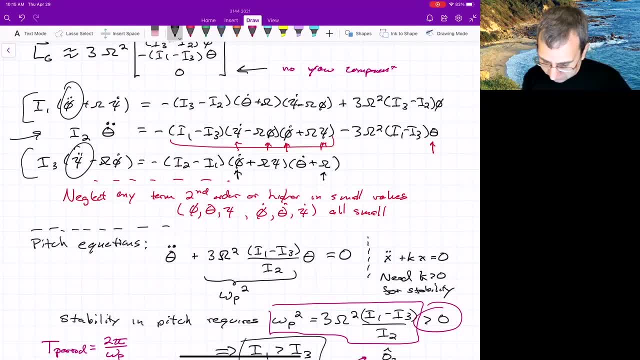 have terms here like this thing will multiply times omega and it'll be just first order and something small. And then this thing will multiply by this And again give us something first order and it'll be same thing up here. So these terms don't just go to zero And then over here. 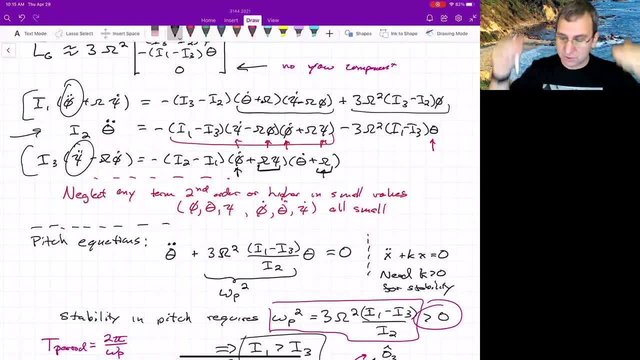 we got something else going on, All right, So we'll collect those two terms. So this is the, the roll and the yaw. You notice that they are coupled, So the dynamics in roll and yaw depend on each other. Pitch was decoupled. 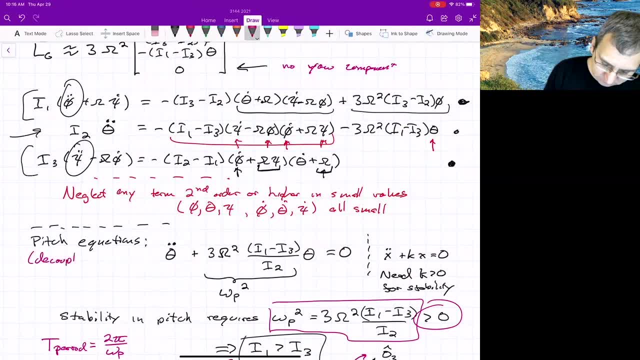 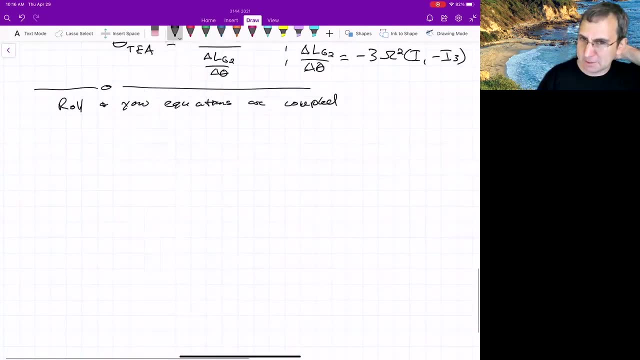 from them both. So pitch equations, at least for small deflections away from equilibrium, are decoupled from roll and yaw, And then roll and yaw become another problem for us, because they are coupled, And if you collect them into a form that is, 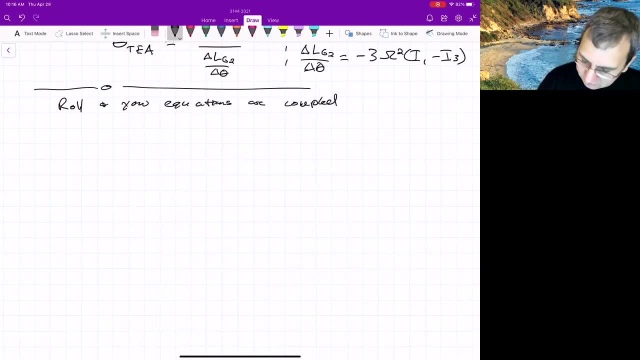 amenable to analysis, you will get something- And this is just the linearized ones, right Linearized- Dropping all terms that are second order and things that are very small, You'll get roll, double dot, yaw, double dot plus, And now we've got a two by two matrix, zero, omega. 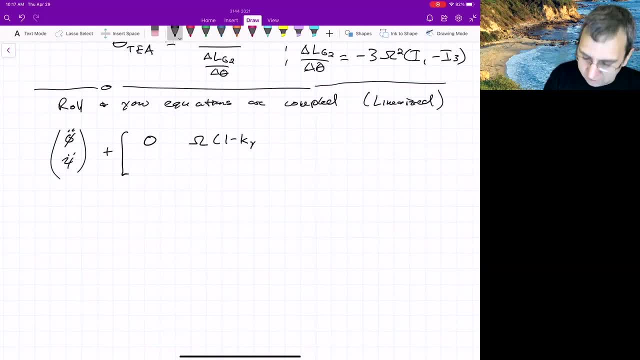 one minus a new thing that I'll define as ky, And then over here it's omega kr. They're kind of like effective stiffnesses And this is what the literature uses. This is times, v, dot, psi, dot, The inertia ratios that we use. kr is i2 minus i1 over i3.. Ky is i2 minus i3 over i1.. 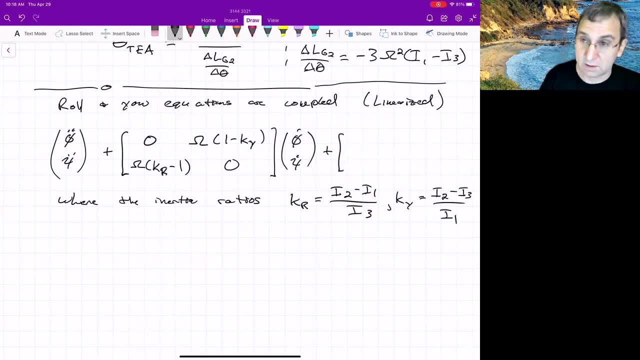 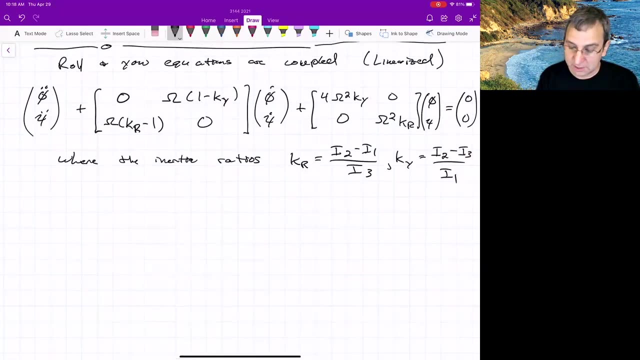 We haven't yet finished this. Then we have another two by two, for omega squared Ky is zero. omega squared R: This is times, roll and yaw, This is moving over, And this just equals zero. zero To study the stability of something that's coupled like this: I don't know if this was covered in dynamics. 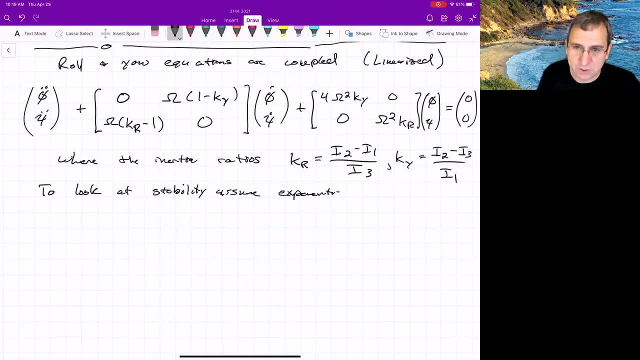 and control. but we can assume an exponential solution. So we're going to assume that phi as a function of time and psi as a function of time are- they've got some initial conditions, times, an exponential, And then we plug that in to these coupled ODEs. 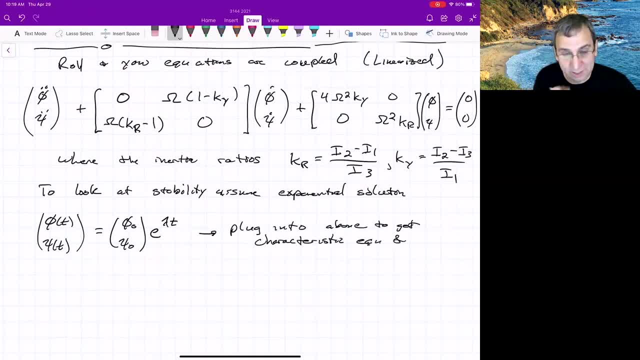 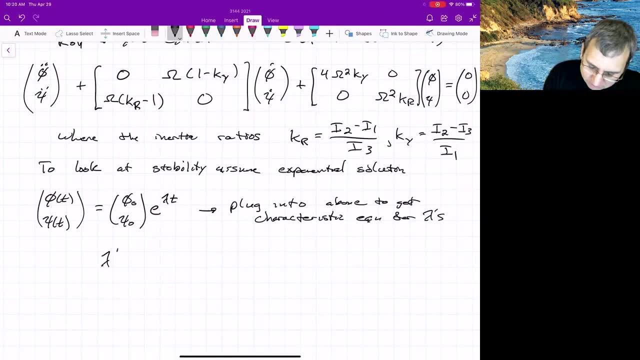 And we'll get a characteristic equation for what the lambdas are. Looks kind of like an eigenvalue problem, But what do we get? We get lambda to the fourth, plus lambda squared omega squared one plus three, ky plus ky, kr plus four, omega squared ky- kr equals zero, And 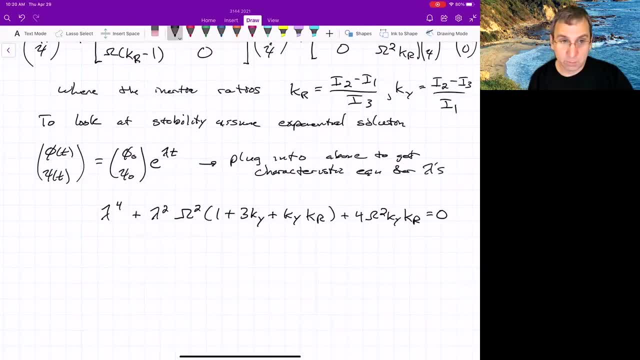 this looks like it's a polynomial, a fourth order polynomial, but notice, we only have lambda to the fourth and lambda squared. If we let x equal lambda squared, then this can be rewritten as x squared plus. let me move this down: b1, x plus b0 equals zero, And then it's a really simple formula that we could solve. 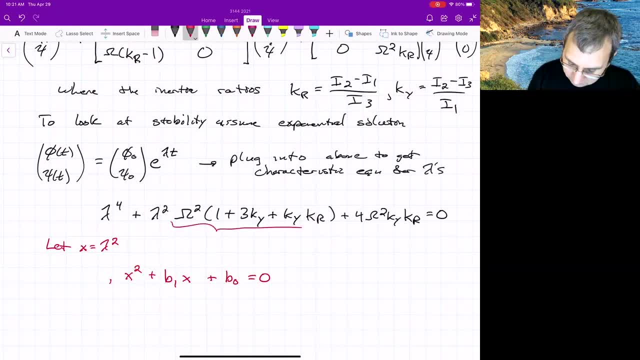 with the quadratic equation. So this term is what we mean by b1, and this term is what we mean by b0. So you can solve by the quadratic formula: x equals one half minus b1, plus or minus square root of b1 squared minus 4b0.. Now we need to check which conditions guarantee that no root of this. 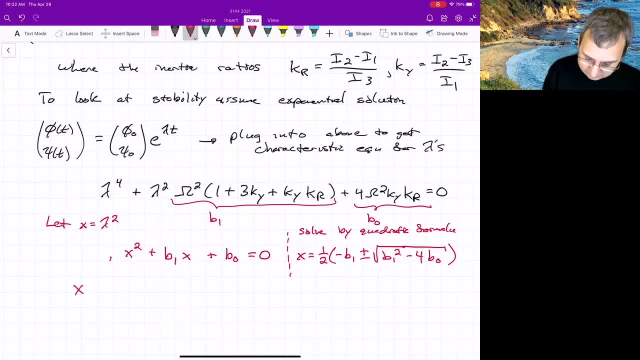 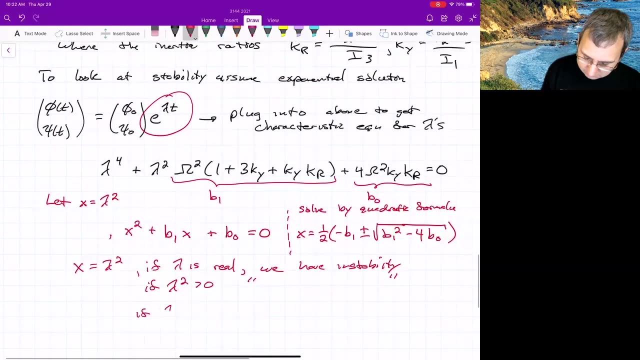 has positive real components. So the solutions will be: x is lambda squared. We assumed an exponential up here. If lambda is real, we have instability. So that means if lambda squared is greater than zero, we have instability. However, if lambda is complex, that means lambda equals, like an i. 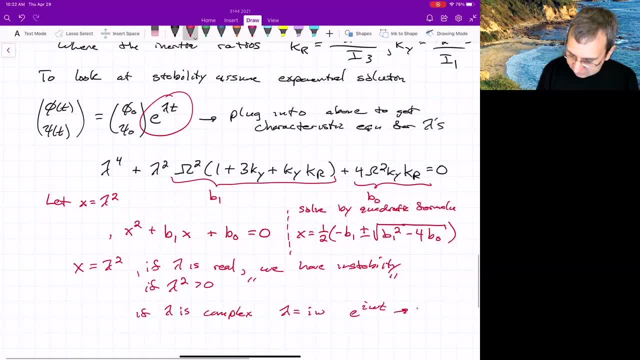 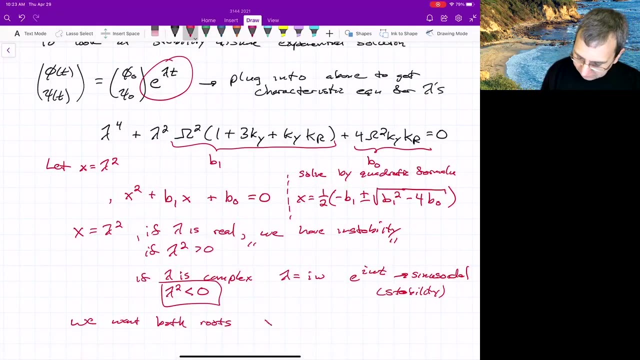 omega, then e to the i omega t is actually sinusoidal and that's stability. If lambda equals i omega, then that means i is not. it's not stare. Any last questions means lambda squared is less than zero. So this is what we want. That means we want both roots of x. 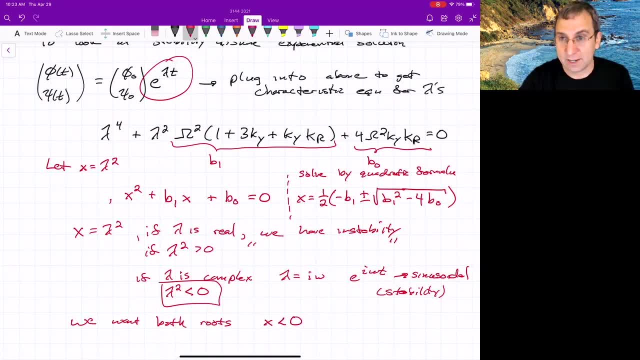 to be less than zero And we can check for that. You could write it in terms of what the signs of b, b1,, b squared minus 4, b naught, but all of those have to be The conditions for both roots. 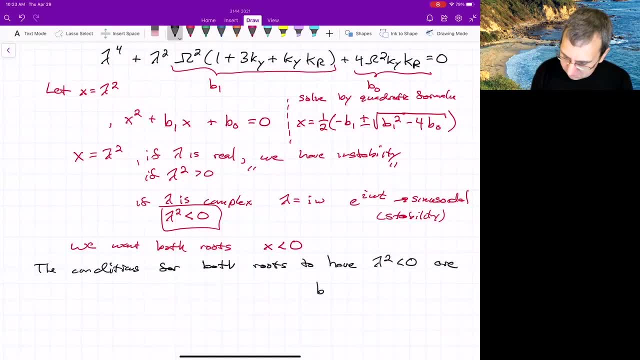 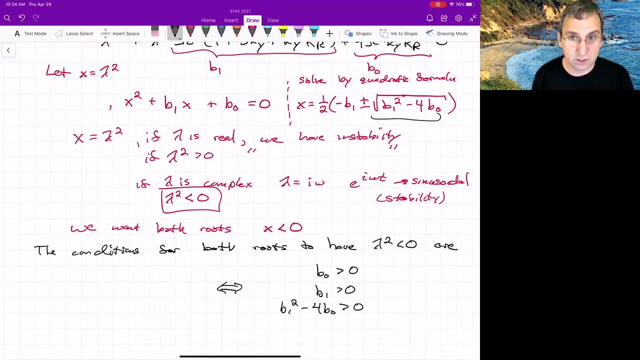 to have lambda squared less than zero are: b naught needs to be greater than zero, b1 needs to be greater than zero. b1 squared the thing inside that square root minus 4, b naught needs to be greater than zero, And all of these can be written in terms of those ratios, kr and ky. So this is: 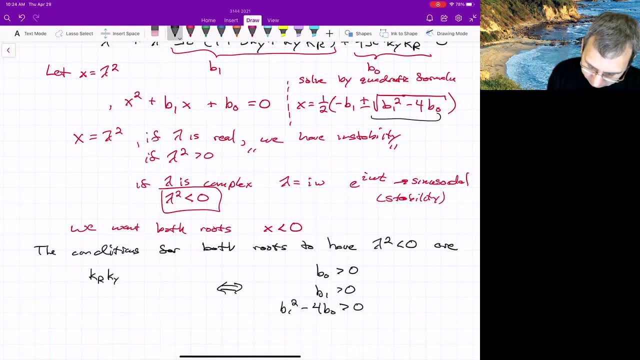 equivalent to krky is greater than zero. 1 plus 3ky plus krky is greater than zero. And this other one is pretty weird: 1 plus 3ky plus krky squared is greater than 16kykr. Also, from before, ky needs to be greater. 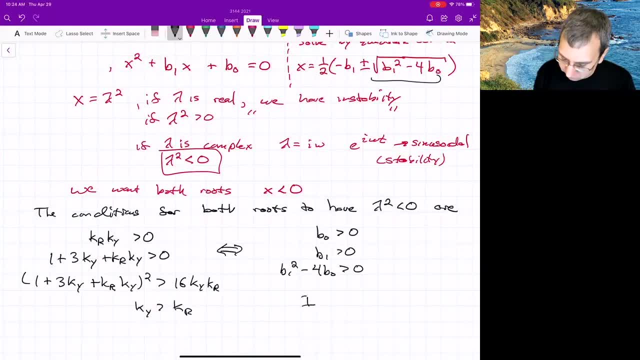 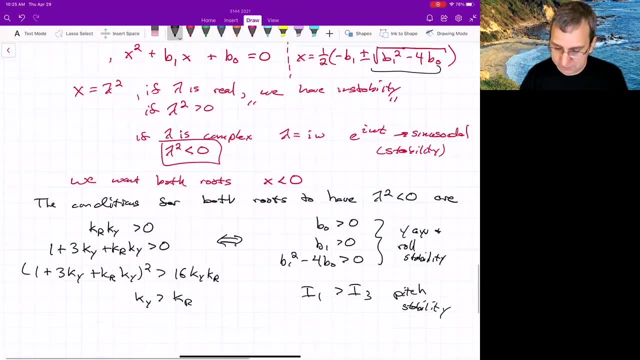 than kr. That's equivalent to what we already had from before. This was the pitch stability. We want everything to be stable, So this is for yaw and roll stability. If we have that, then we'll have what we want. It means that I 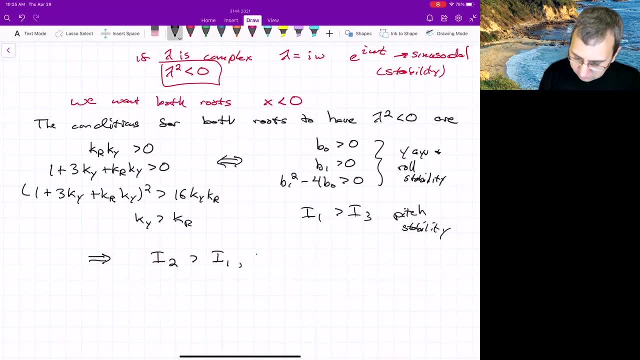 I2 is greater than both I1 and I3, or I2 is less than I1 and I3. And we already know how they're related. So if we have that, then we could write down what the frequencies are, And it's not like. 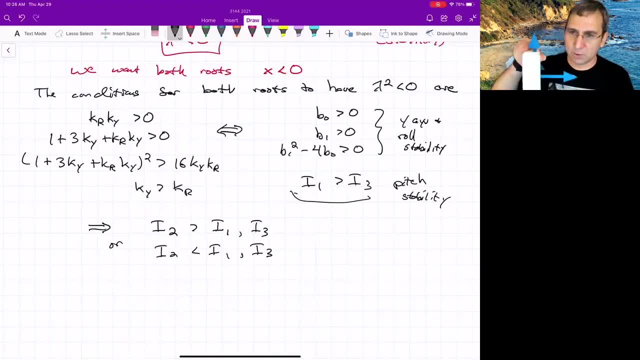 there's because yaw and roll are coupled. it's not like we're getting a frequency for roll and a frequency for yaw. They're both coupled. So if we have that, then we could write down what the frequencies are. So if we have that, then we could write down what the frequencies are, And it's not like 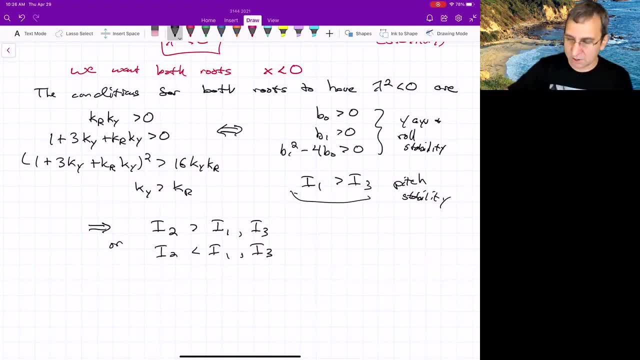 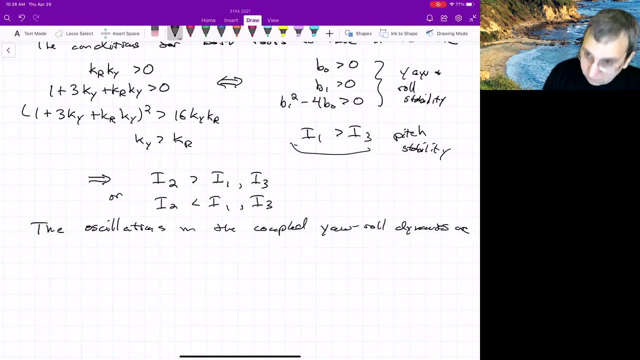 they're coupled and they might be moving in some kind of interesting way, But there are still two frequencies. So the oscillations in the coupled yaw-roll dynamics are: if I look at those roots up above, I'd call them omega 1 and omega 2 are square root, negative lambda 1, 2.. So this just 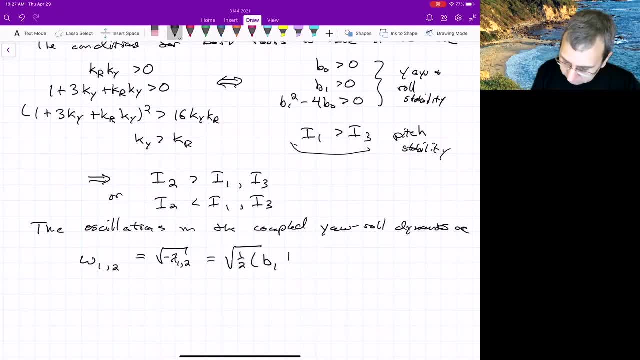 means square root of one half b1 plus or minus square root of b1 squared minus 4b0.. We could also summarize the yaw and roll dynamics. So if I look at those roots up above, I'd call them omega 1 and 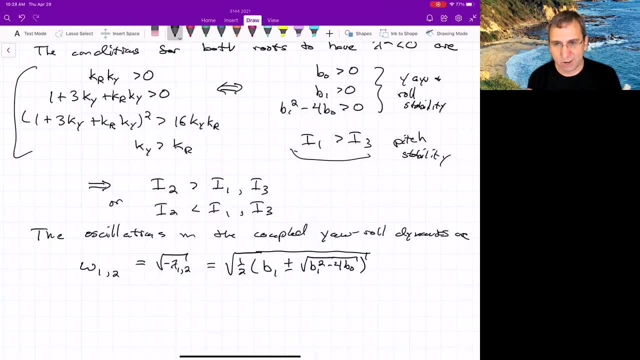 omega 2 are square root of 1 plus 4b0.. So these conditions over here in terms of a diagram, you could call it the gravity gradient stability chart, where we're just looking at the regions in kr ky space, those two parameters that lead to stability or instability. Let me show the 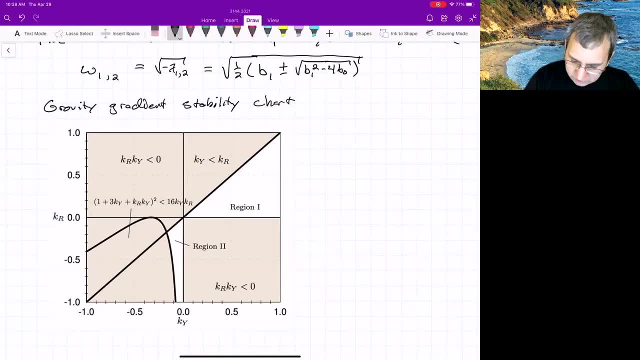 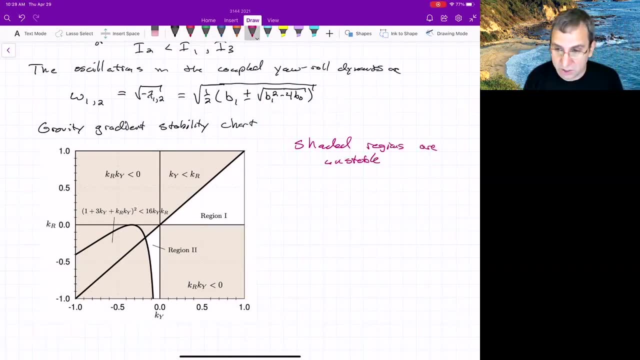 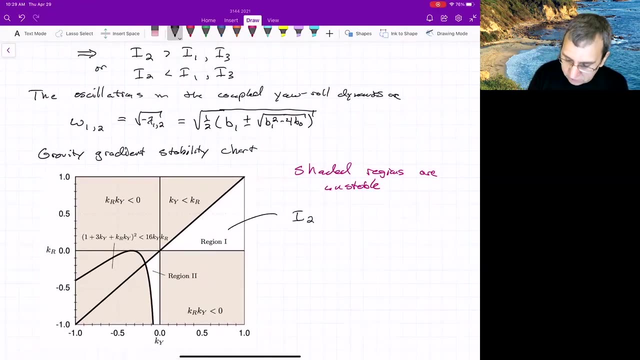 gravity gradient stability chart. The regions that are shaded are not good. They're not stable. Shaded regions are unstable. Regions that are unshaded. there's two of them and they correspond to those two conditions up above This one called region one. this is where I2 is greater than I1, which we already know is greater. 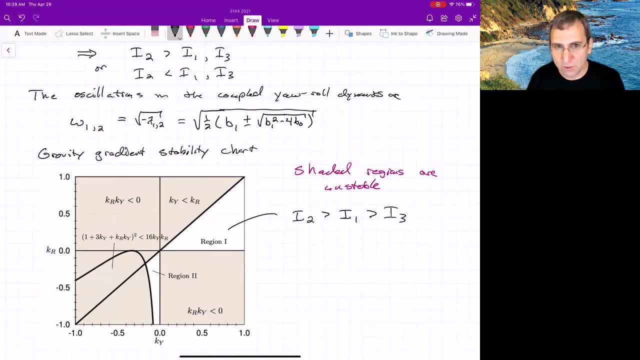 than I3. So that means the moment of inertia along the I2 direction. that's the one normal to the orbital plane. that's the largest moment of inertia. This is the one that's commonly used. It's commonly used because, due to kind of nonlinear effects that I can't really go into, 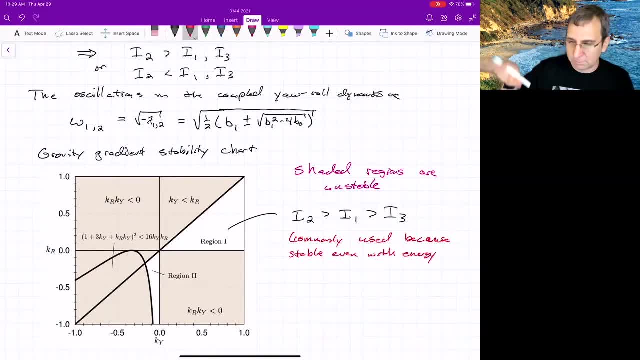 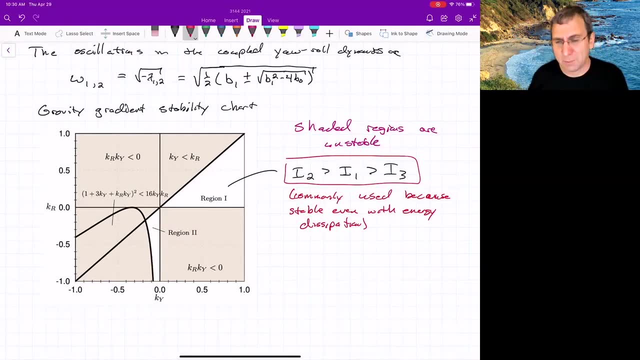 it's stable even when there's energy dissipation due to vibrating parts of the structure. That would be the condition for stability that I want you to look at The other one. it's unstable when you add energy dissipation, for reasons that are complex, But this one has. 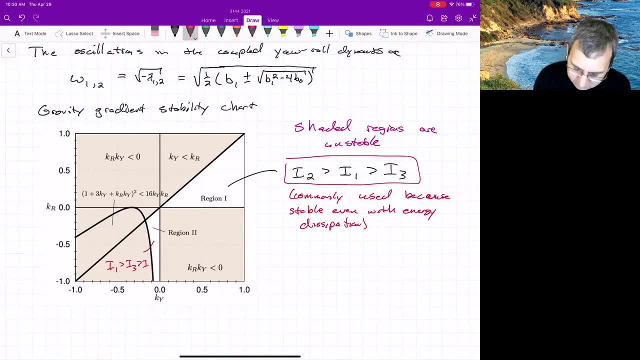 I1 is greater than I3, and it's greater than I2.. So I2 is actually the smallest. So maybe we just hash that and say kind of unstable, don't use Due to vibrating parts of the structure, it will go unstable. This one is called the Lagrange region, which is fun, I think it must. 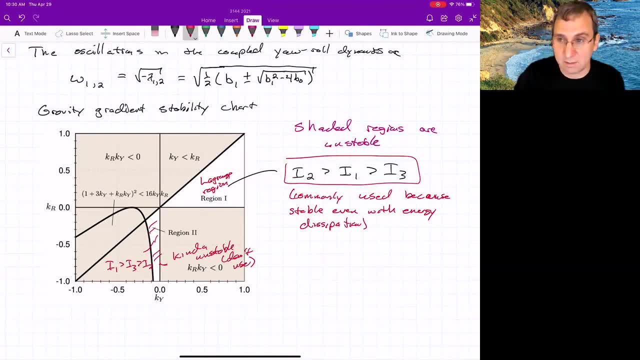 have been Lagrange? who did an analysis like this? I honestly don't know. So that would be the condition. So if we had this thing, and let's call the orbital direction that way, This is the stable configuration. Your phone. Your phone is easy because it's got the 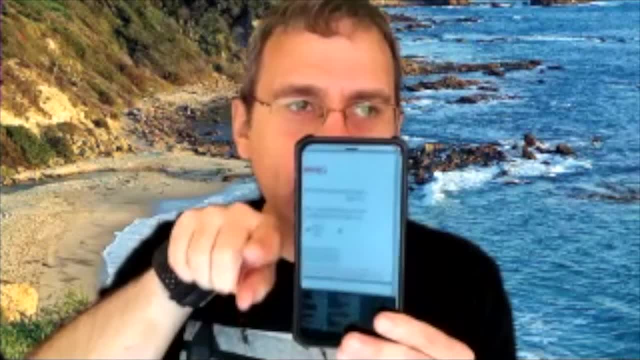 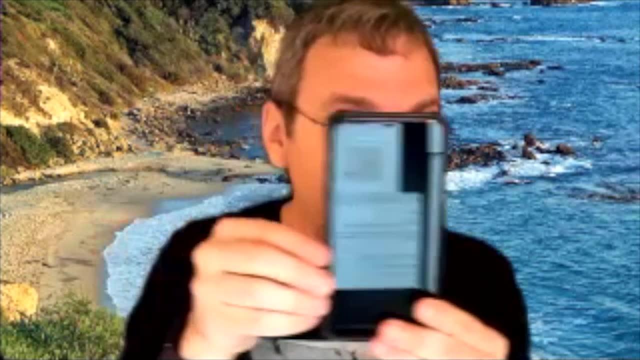 largest moment of inertia through this way. And this is the orbit normal. So coming out of the screen, that's the orbit normal. And then I1 is actually the intermediate axis. So this is actually going along from the intermediate axis, this iPhone, So phones going through space if they. 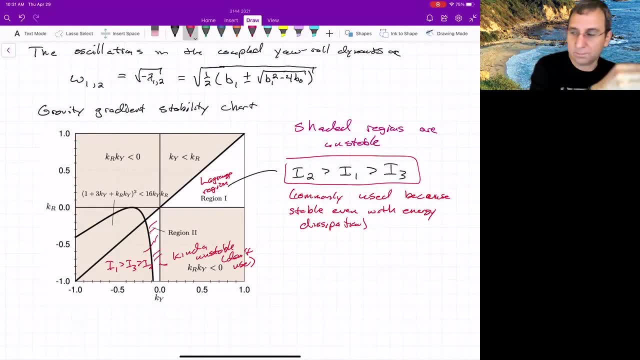 are unstable, gravity gradient stabilized. they'll go this way. Excuse me, Professor. Yeah, So I know that we refer to bodies like this as unstable when k is less than zero And as stable when it's greater than zero. What do we say? it is when? 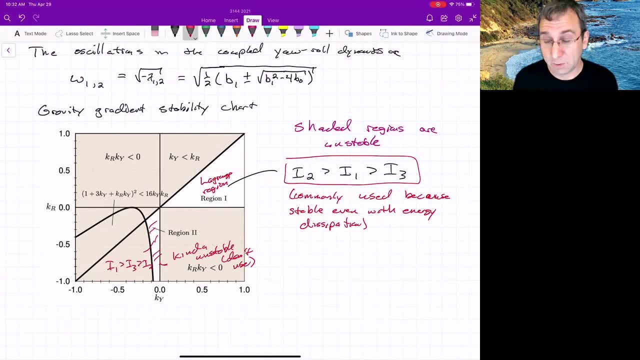 it's equal to zero. We would say it's neutrally stable, Yeah, So, yeah, that's why I'm making these qualities greater than or equal Plus. you're not likely to have that situation right. This machine precision won't even allow that. Yeah, I guess you're thinking what if theta double dot? 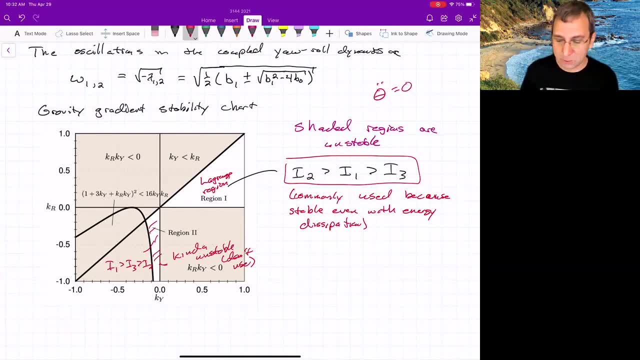 is just equal to zero. That means there's no oscillatory motion, And it probably means that that's just zero times the linear term, And there's going to be some second order term- I don't even know what to call that. It's going to be something that will dominate, And so that'll lead to some nonlinear dynamics. 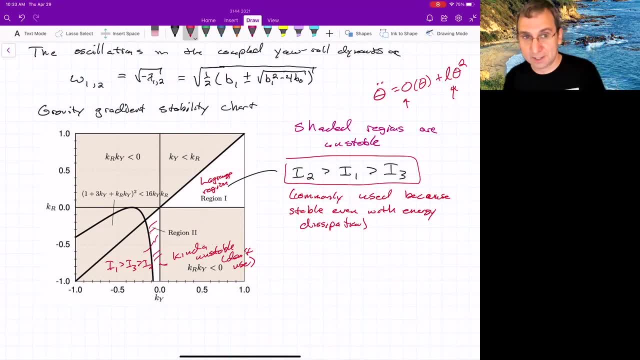 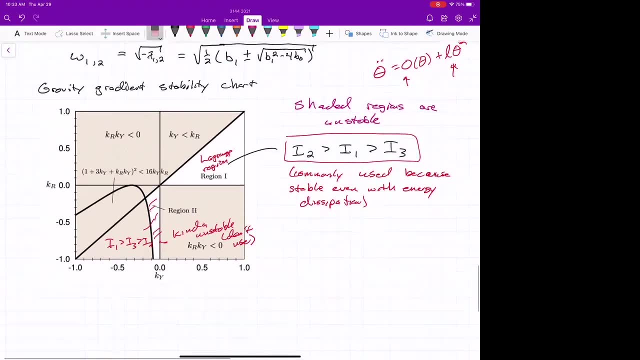 So you're thinking of just the linear term goes away, but then there's all the nonlinear stuff which you would then have to look at. Does that make sense? It does, Thank you. I just want to ask a quick question: Are these equations we derived? 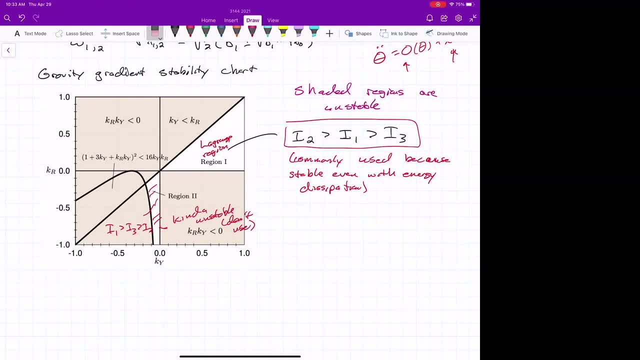 are they only valid for the three two one that we started with, Or are these- I guess the second half- all generic? We used the yaw pitch and roll to get at this, But this is this is true, independent of how you look at the kinematics. We just used the yaw. 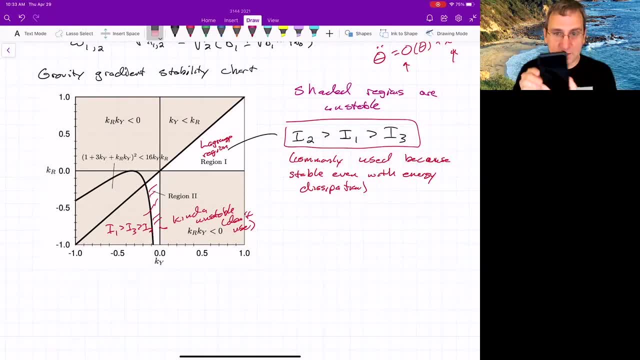 pitch and roll for convenience. Okay, thank you. The phone going through space this way is going to be stable, no matter how you think about it. So I thought in the last little bit we could talk about an application of this. It's a. 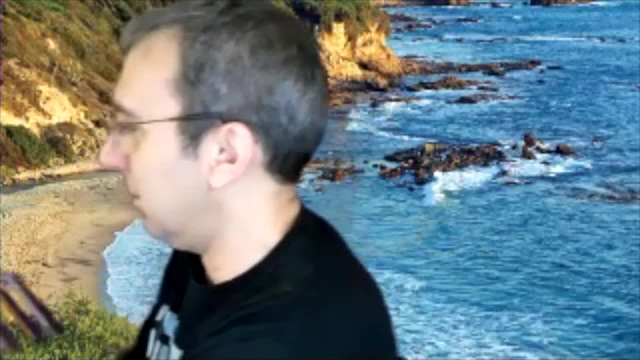 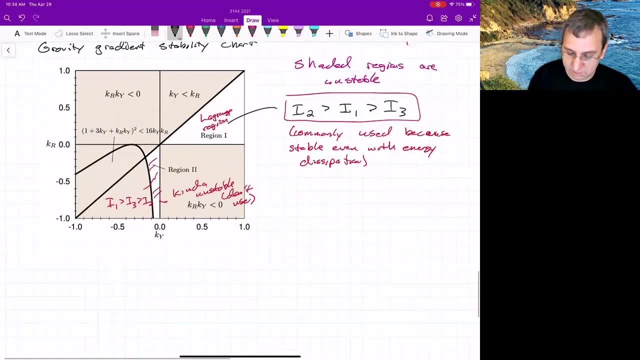 Space Station like: look at this, Oh my goodness. It's made up of so many parts And they all have their own moments of analysis inertia. Let's try this on the International Space Station. First of all, is it near an equilibrium condition and is it in the stable one? You know what the space station looks like. 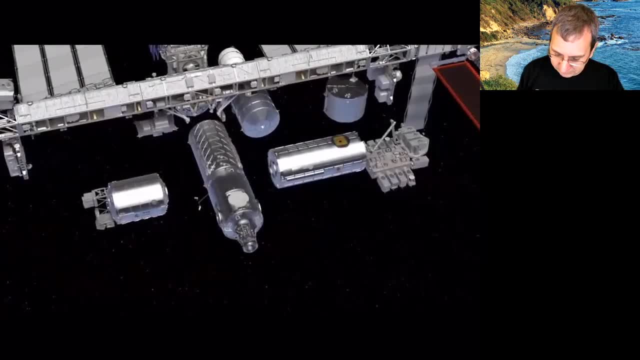 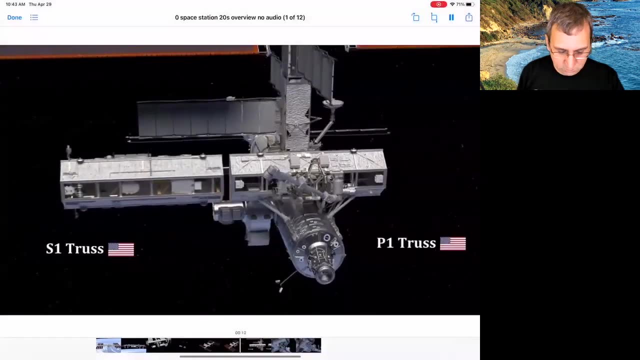 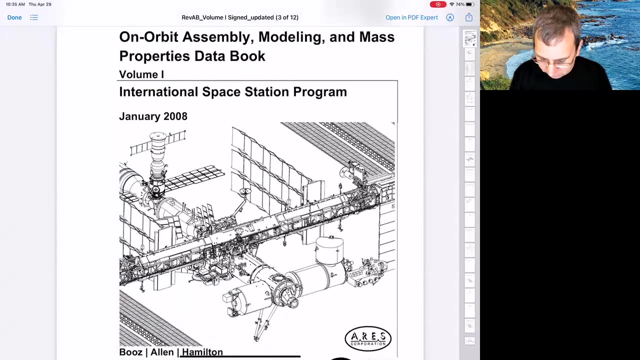 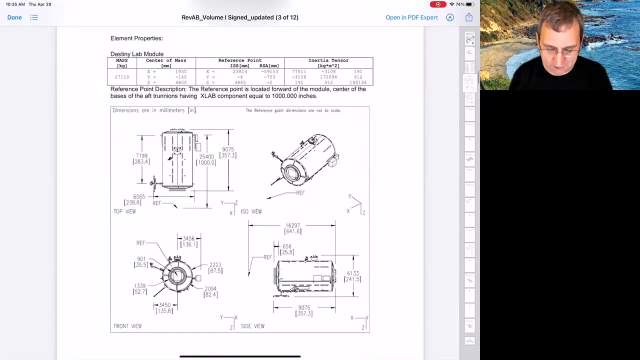 It looks like this. Check it out Now. there's this whole video that somebody made of putting all the parts in- Pretty neat. There's all this documentation about the space station. so this is a handbook of what the space station looked like in 2008,, and it's got all these things about the parts, all the details. 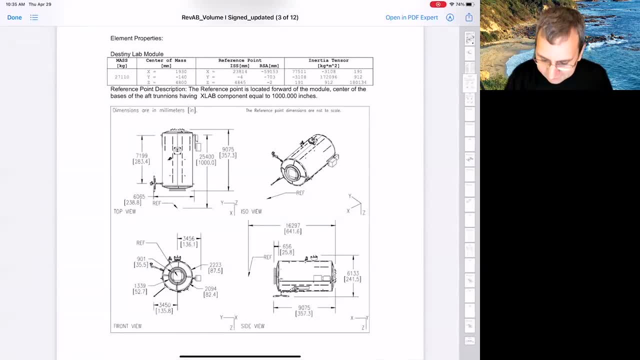 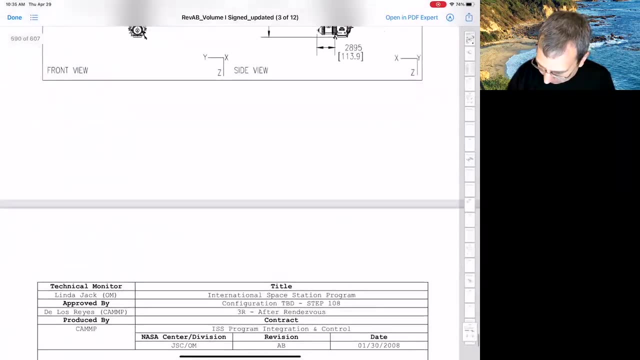 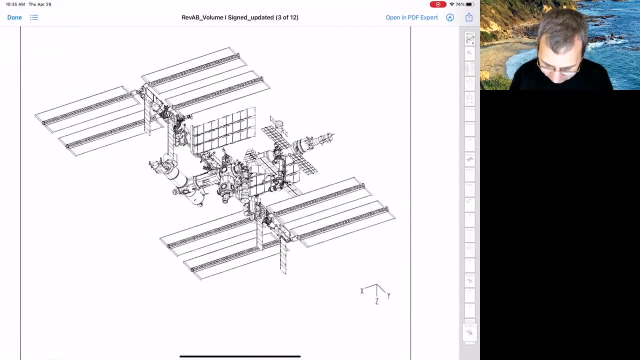 of every part, including the inertia tensor, and they've also set up what the reference frame is for us. Is this the one that I like? Yeah, I think I like this one. I really don't like this drawing. It's kind of lame. The spacecraft is going. 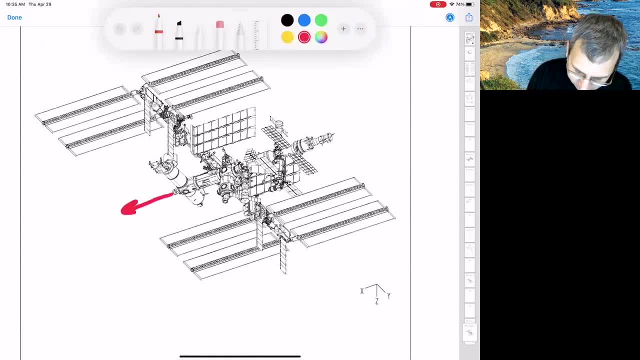 in this direction, That's the orbital direction. so that's what they're calling x, x. And then there's down, They're calling that z. And then let's see, to complete the right-handed coordinate system this way is y. So that's what they've set up as their coordinate system and I think it basically. 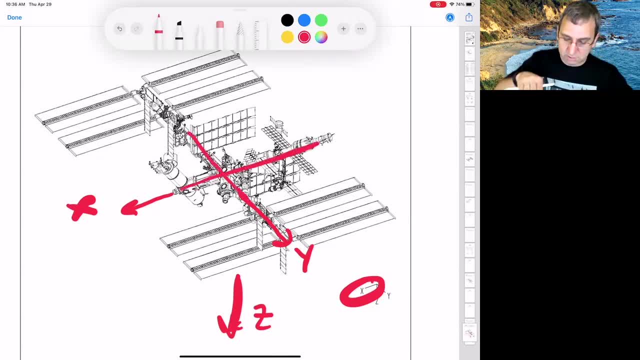 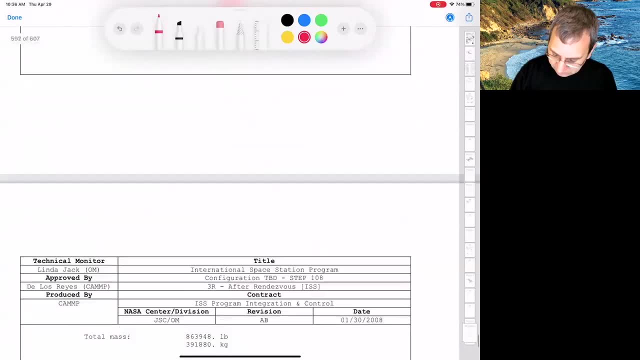 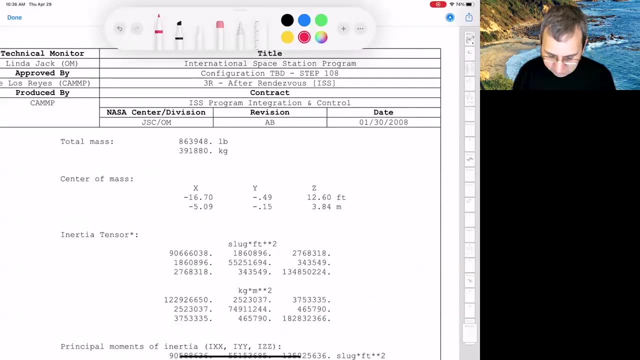 aligns with these directions of the structure, but those aren't necessarily the principle axis directions. To get to the principle axis directions you need to do some more things. So it says for that configuration up above like: here's the total mass, here's where the center of 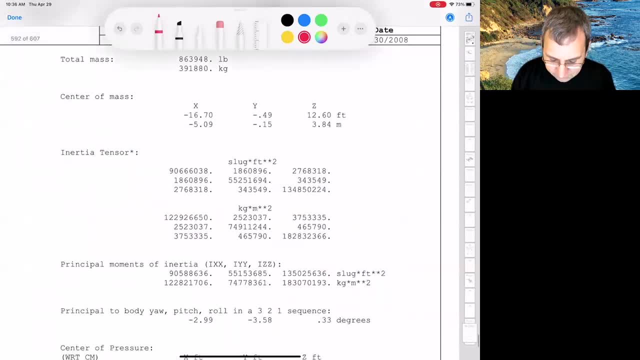 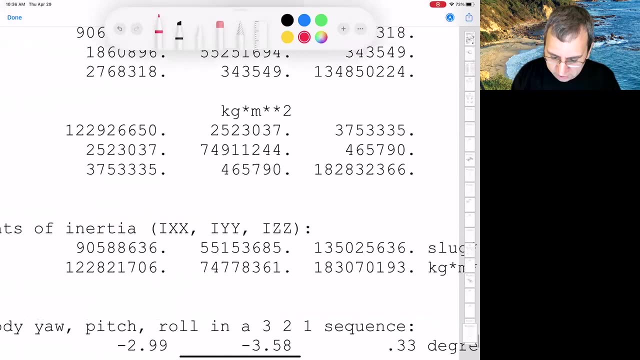 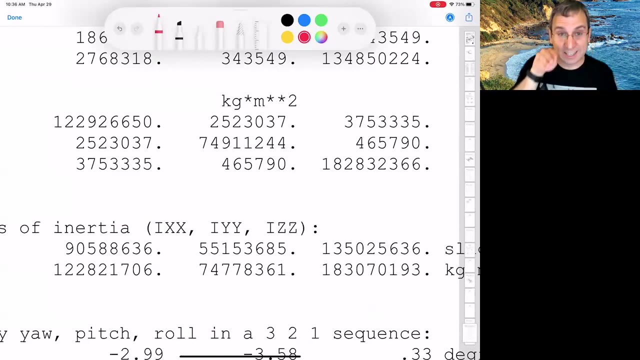 mass is with respect to something. and then here's the inertia tensor, And forget about slug per. you know square feet. Think metric, Otherwise things will start crashing. Just please do metric. So this is the moment of inertia tensor with respect to that: x, y. 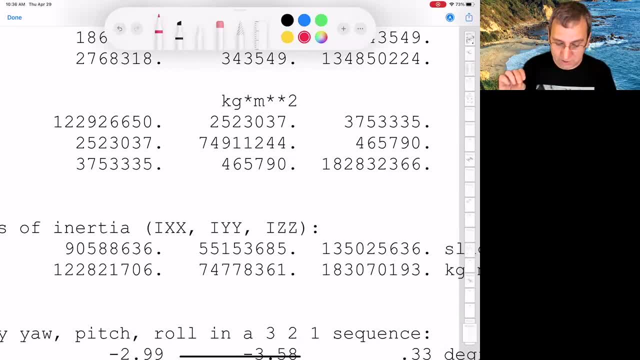 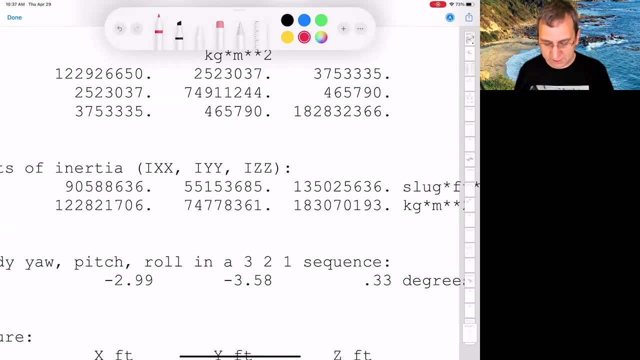 z body fixed frame on the space station. And look, they've even already calculated the moments of inertia. And then what the yaw pitch and roll sequence is. it's different from the yaw pitch and roll that we defined. They're doing z down. okay, You can see these are in degrees and it's very 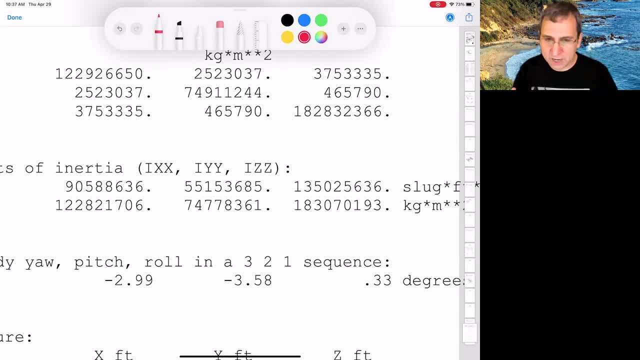 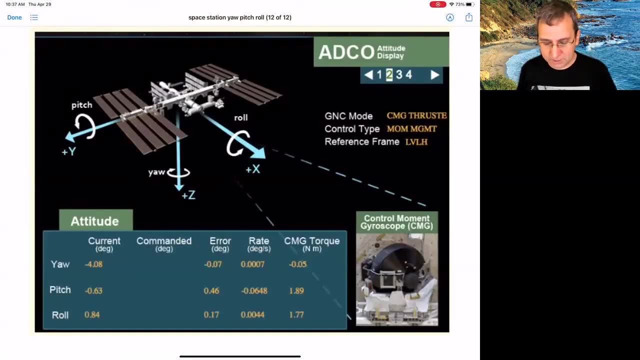 small, So the x, y and z are pretty close to the yaw pitch and roll. So this is showing the space station as it's moving through. how they've defined x, y and z. They've got this control moment gyroscope And you might go. well, why do they need that if the 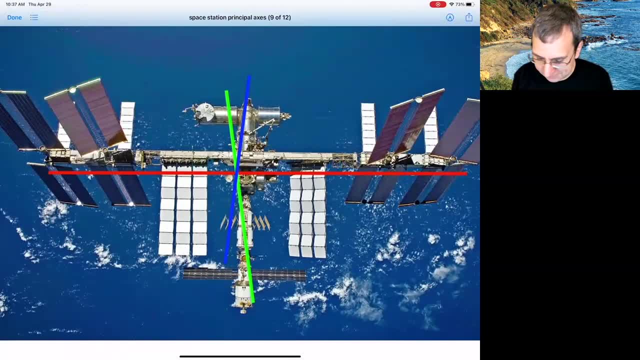 gravity gradient's stabilized If you were to color in those axes. we've got some principal axes here And you notice they're not exactly aligned. So that green one isn't exactly aligned. So that's the principal axis. Is it the intermediate right? This is the direction of the orbit. If I were to 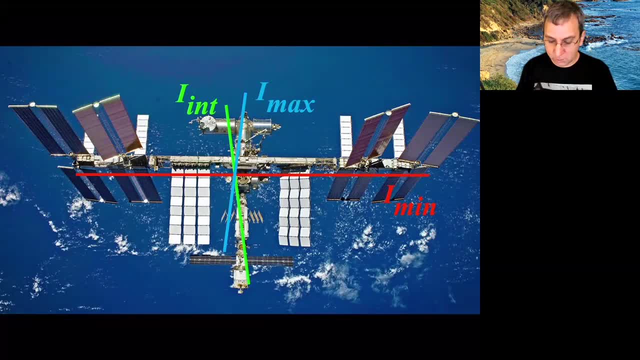 label it. I get this. So the direction of the orbit is the intermediate axis, which is good. I said that was good. But the local vertical is actually I max And it's supposed to be I min for this to be in the gravity gradient stabilized attitude. So it's not stabilized, It is at an 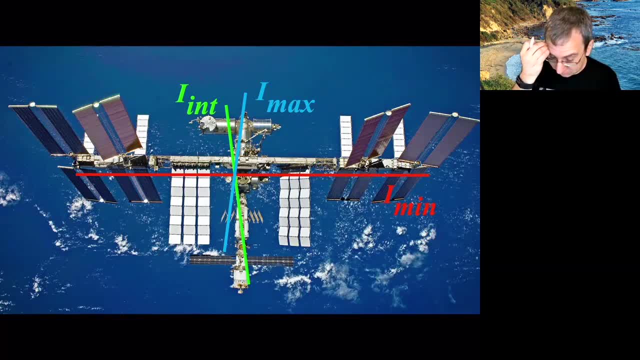 equilibrium. It's just at an unstable equilibrium. That's why there's that control moment gyroscope. It's good to be near an equilibrium because just with a little bit of torque you could stabilize it, But that is why they have that. Plus, the space station violates some of the assumptions. 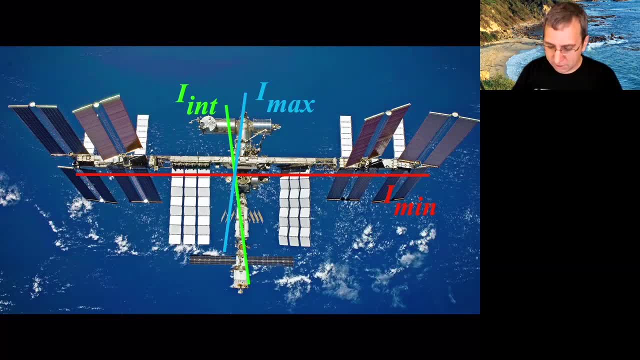 we made, Which is that we have a rigid structure. There are whirling gizmos, There's also people walking around and bouncing off things, There's the panels moving, So there's a lot of motion on this thing. It is not perfectly rigid, And so that's why you would need a control moment gyroscope. 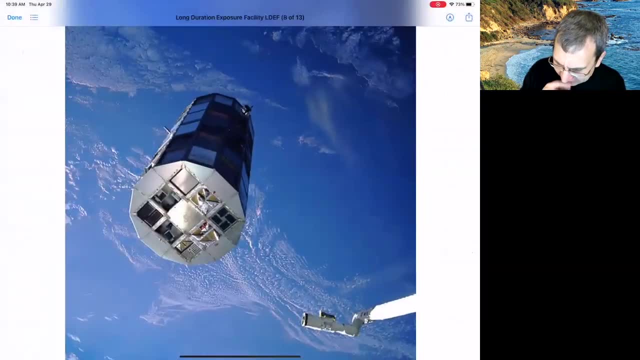 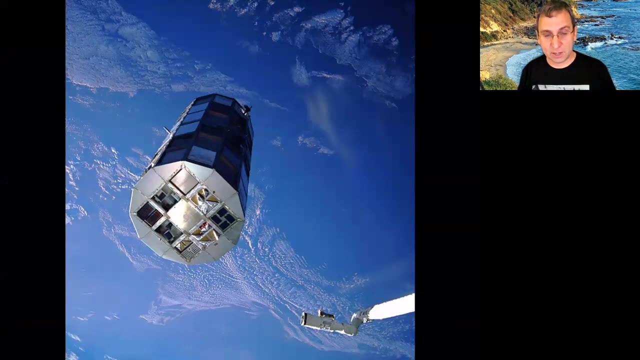 We'll get back to the space station. There was something launched I think in the 80s. It's called the Long Duration Exposure Facility, Roughly a bus-sized thing, And it was gravity gradient stabilized. It was put out by the space shuttle. 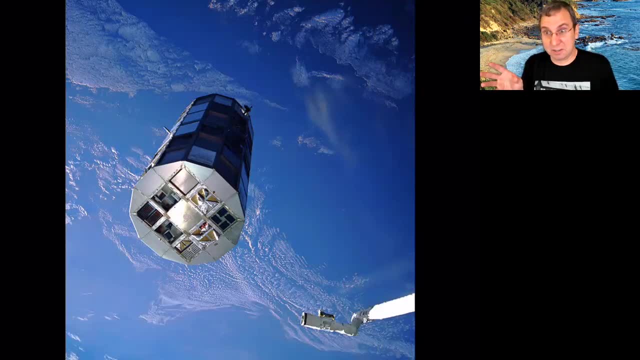 There were a bunch of things that were going on. There were experiments on it And they left it out there for, I think, several years And then collected it again. It's kind of cool And you can see it's. maybe it's hard to see, it is. 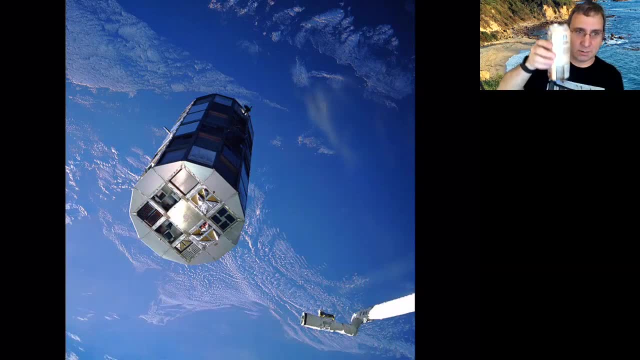 pointing up and down like this can. It's got its long axis, So the minimum moment of inertia axis, aligned with the local vertical. So if it had even a little aerodynamic torque or something, it's stable. Might wobble a little bit, but it's stable, It's not going to flip, So that's good. 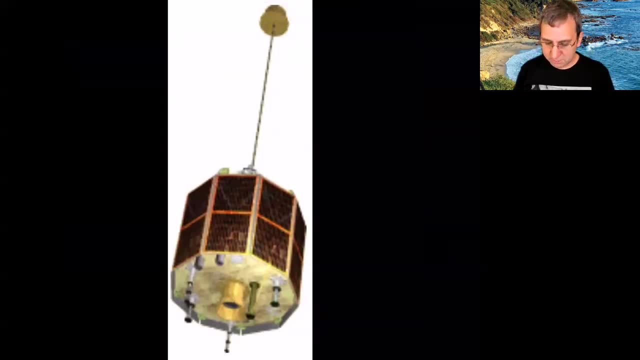 There were others. You can put out a large boom. This isn't very big, This is like as big as a trash can. But then they put out this long kind of rigid thing and a mass at the end. This was. it's called OUSAT. 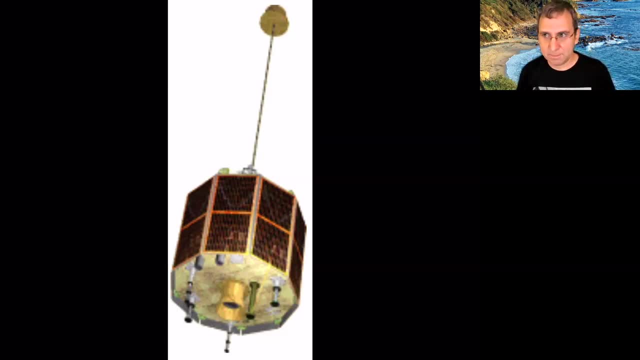 University of Surrey satellite. There's this university in England that I've been to And it's kind of like they've got this mini JPL that puts up little spacecraft for Britain and all kinds of different countries. You just want to have a little spacecraft up there And they used. 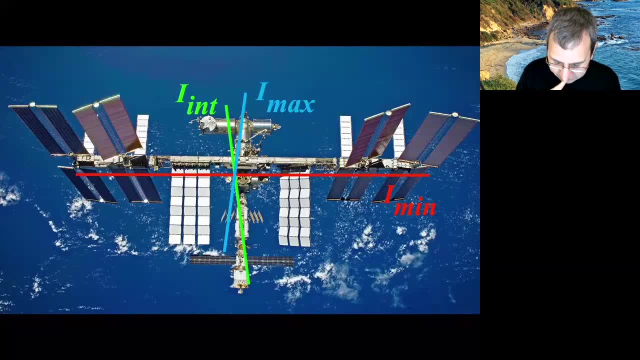 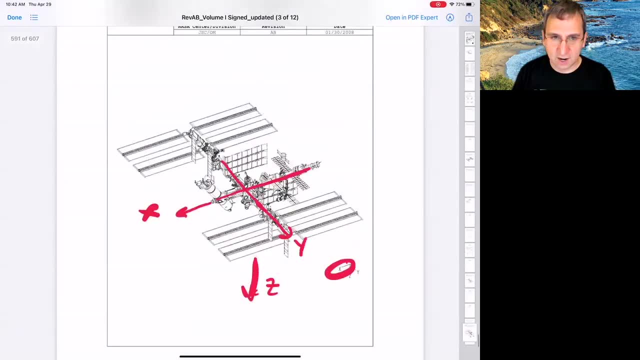 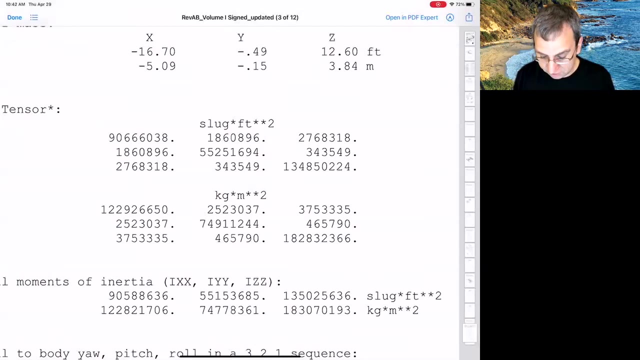 gravity gradient stabilization. We can calculate things for the space station. I guess, if we wanted to, They have to figure out the moment of inertia for all kinds of different configurations, When something's docking, when the panels are going full blown. So here's the inertia tensor for just one particular configuration. You. 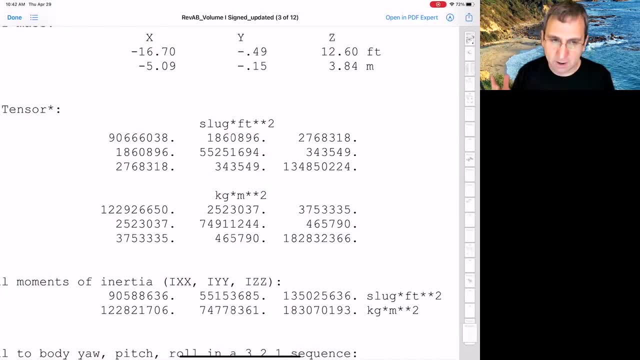 could just read off of here: The things along the diagonal are at least an order of magnitude greater than the off diagonal elements. So that means the X, Y and Z that they have are pretty close to the principal axes And I'm sure that was by design. What's the largest? The Z, And we said for it to be gravity. 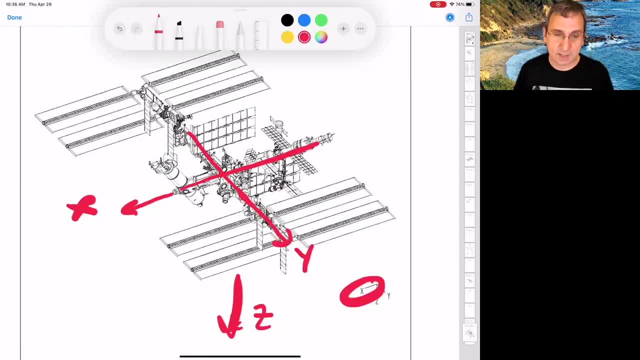 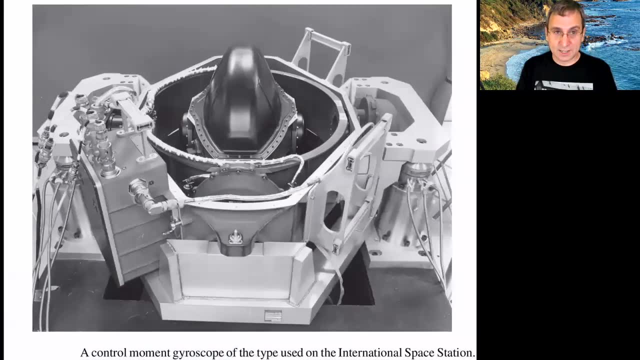 gradient stabilized. that needs to be the minimum, But it's not So. that's why they have that control moment gyroscope. The control moment gyroscope. it's big As this thing turns inside that black casing is a flywheel And it is massive And this is near the center of mass. So as that thing turns. 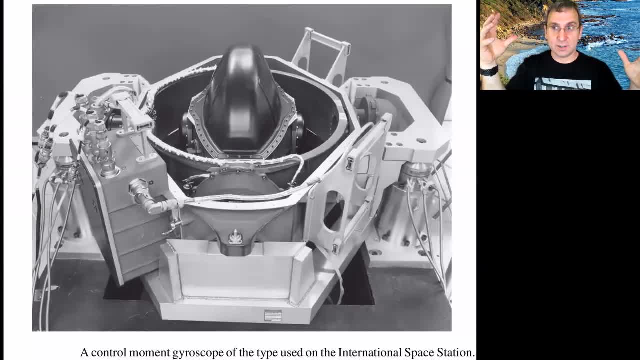 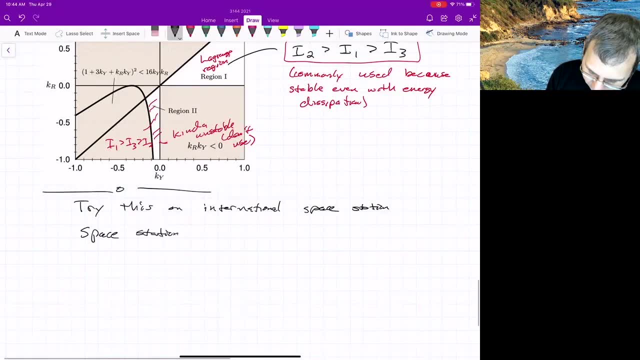 to conserve angular momentum. the entire craft turns as well. So that's what control moment gyroscopes do And space station. it has its B1,, B2, and B3 parallel to the orbital. I just mean it's parallel to these frames. It doesn't mean these are exactly aligned directions, It just 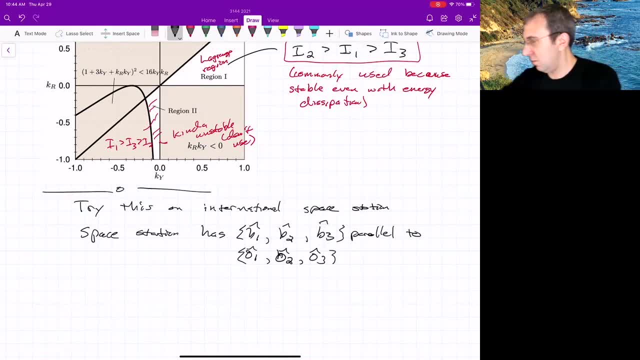 means the frames are parallel. What does that mean? that for frames to be parallel, I might be wondering. Like this is parallel, This is parallel. Even like this is parallel, This is parallel, This is parallel. I mean some direction is either pointing in the same direction or the total.